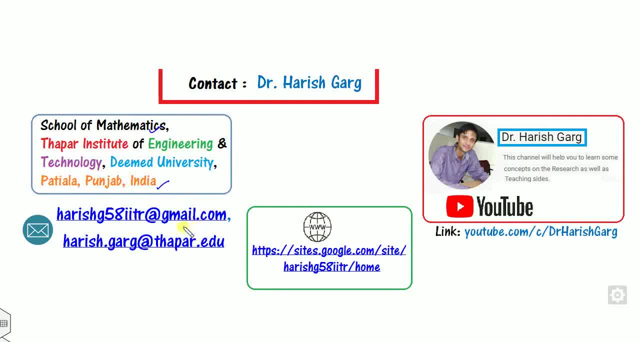 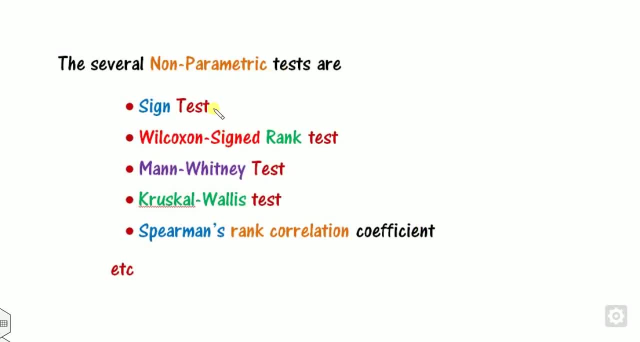 of Mathematics Thapar Institute, India. You are most welcome to contact me by either of my email IDs or through my website or through my YouTube channel for spreading the knowledge. So what we have discussed so far, the several testing of hypothesis- This is the sign test we covered in. 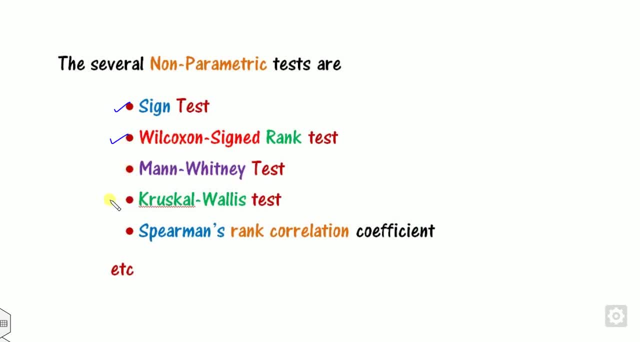 the first class. We will caution. we already discussed about that. Right now we are here, So this, all the others non-parametric testing- we have already discussed and you can find the link of these videos in the description of this, So it must necessarily be discussed. 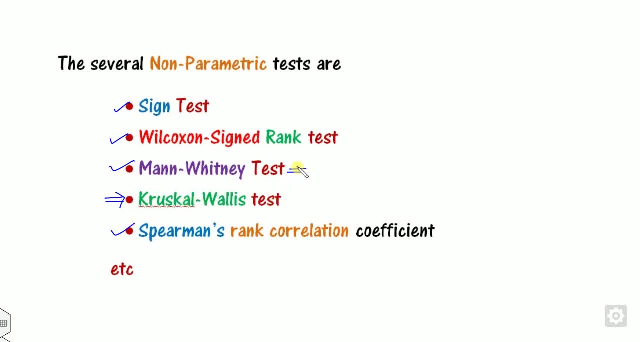 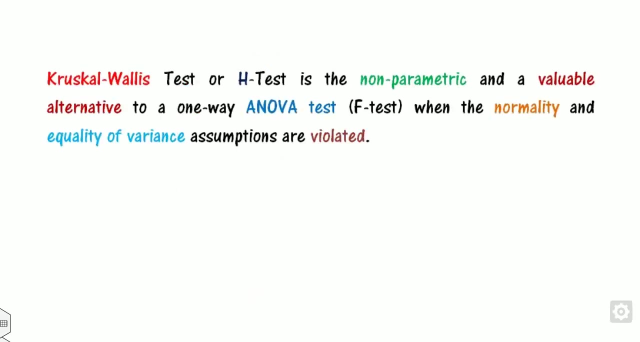 Before watching this video, you must watch the Mann-Whitney test, because it's similar to that of the Mann-Whitney test. It is also called as the U test, and this Crucial Wallis test is also called as the H test. So what is the Crucial Wallis test? So the Crucial Wallis test, or H test is: 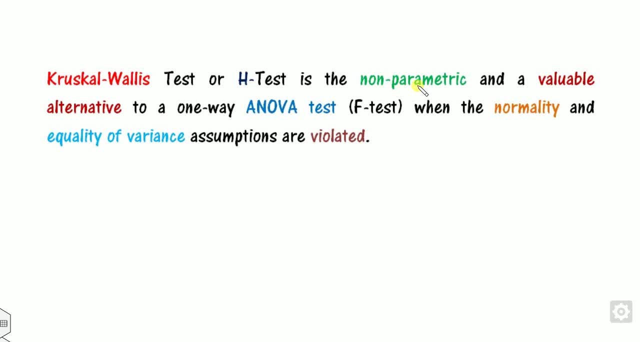 the non-parametric test and which is a valuable, which is very valuable, and it plays an alternative to the non-parametric test. So the Crucial Wallis test is a non-parametric test and it plays an alternative to the one-way ANOVA test. We know that we have studied the one-way ANOVA in our 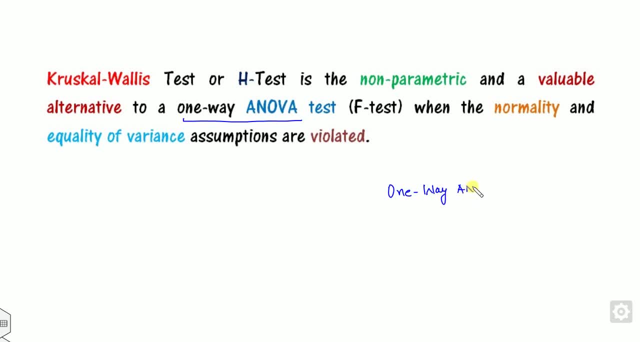 previous lectures and you can see that in our one-way ANOVA what we studied is there is a one classification and we have to analyze their impact, whether there is any significant impact on that. But you must remember that when you apply for the one-way ANOVA, the basic assumption, 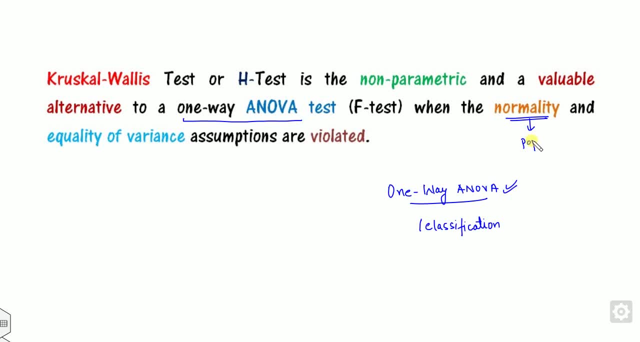 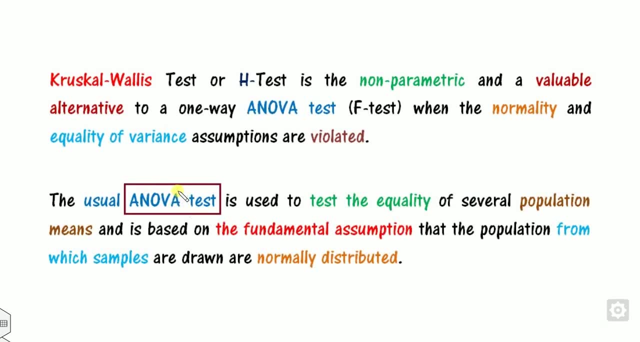 about the normality that is, a population must satisfy the normal distribution and the quality of the variance must be satisfied. But what will happen if this normality test is used to test for the equality of the several population and the basic, fundamental assumption is the: 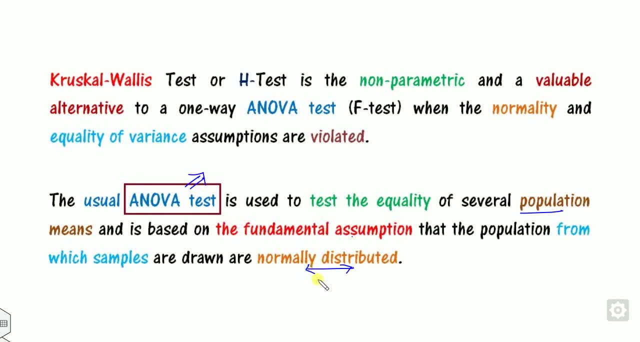 population is drawn from the normal distribution. But what will happen if this condition does not met? then you are unable to apply for the ANOVA test. In an appropriate place of this ANOVA test, we will apply this H test. Also, you have to remember that ANOVA test is applicable only when there is at least how many samples. 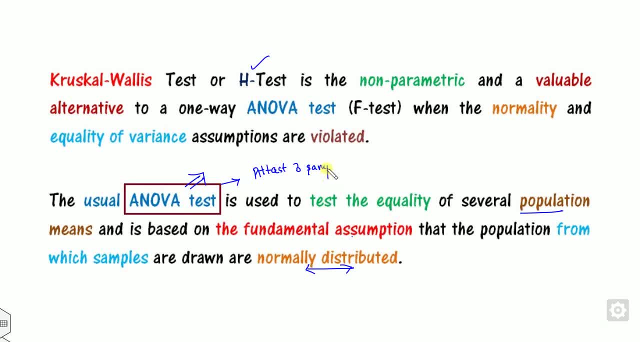 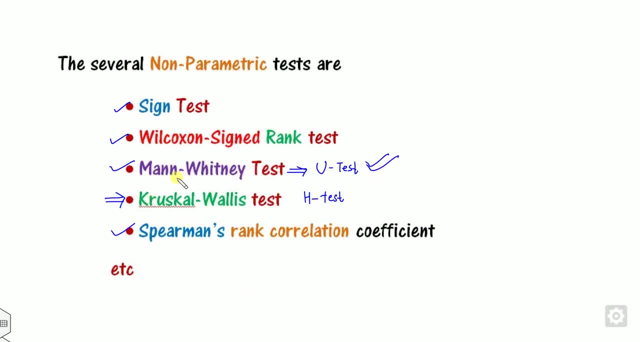 Yes, at least three samples must be drawn. The same thing for here, The crucial wallis test is applicable only when there is at least three samples are there? When there is less than of the three samples, then you can apply this U test, Mann-Whitney test. Okay, so this, what are the basic? assumptions that we have to apply for the one-way ANOVA test. We have to apply for the one-way ANOVA test to get the null hypothesis. So for the one-way ANOVA test we are required to apply the H test or 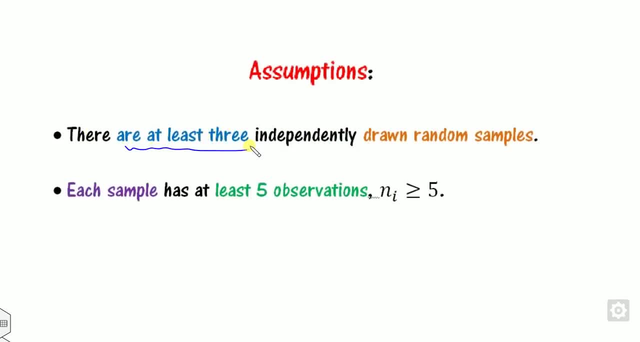 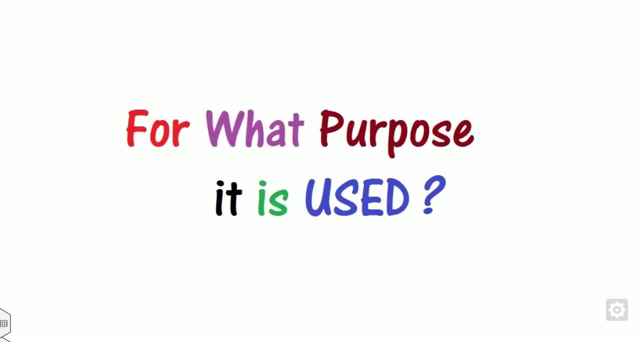 crucial wallis test. There are at least three independent samples you have to do, and each sample must have at least five elements. So if either of the condition is not satisfied, then H test is not applicable. So for what purpose it is used? Why we studied this crucial wallis test, or H test? 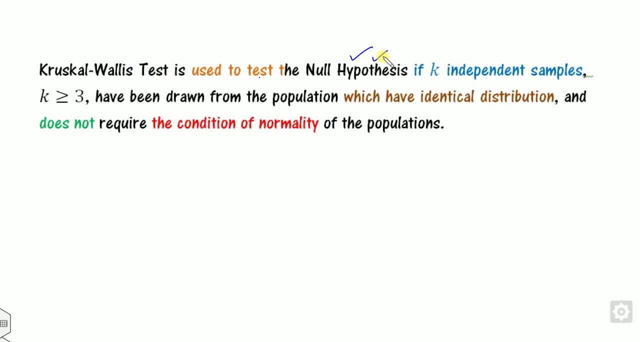 So this test is used to check the null hypothesis that, whether the K- what is the case- It must be greater than or equal to three. The K samples you have drawn have identical distribution or not. That is the basic task and it does not require the condition. 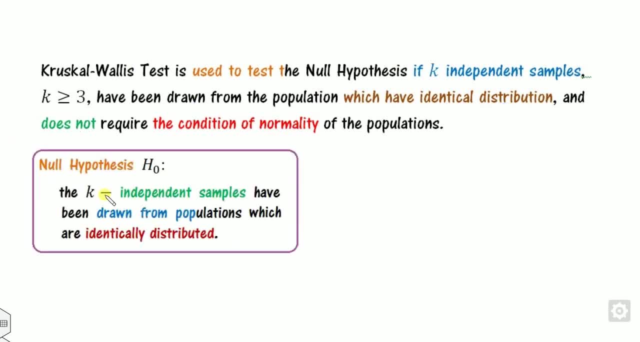 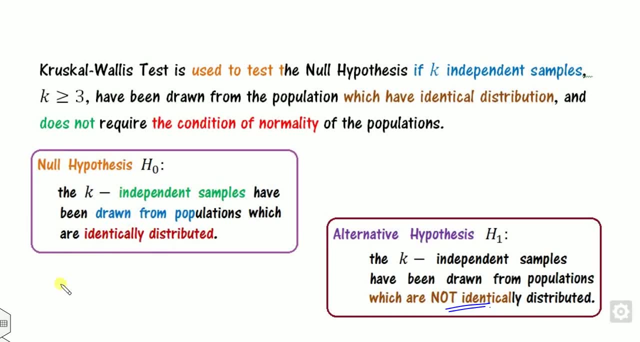 for the normality, In other words, how you write the null hypothesis. is the K samples you have drawn are identically distributed. and what is the null hypothesis? is The K samples are not identically distributed. In other words, in mathematically, how you define the H0? If K samples are identically. 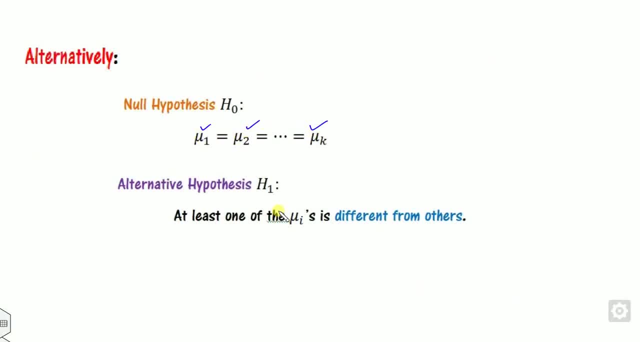 distributed. it means you can write as mu1,, mu2 and muK, And what is the opposite of this is at least one of them. What is the meaning of the? at least is It can be like this way, It can be of. 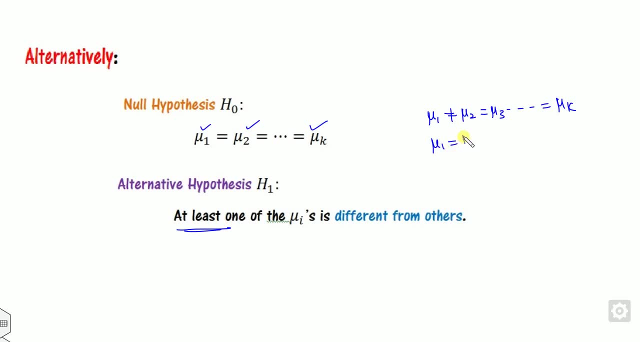 this muK. It can be like this: mu1 and mu2- both are same, but not equal to mu3- is equal to mu4, and so on up to the muK. Or it can be like this way: This is not equal. This is not equal, while all others are equal. 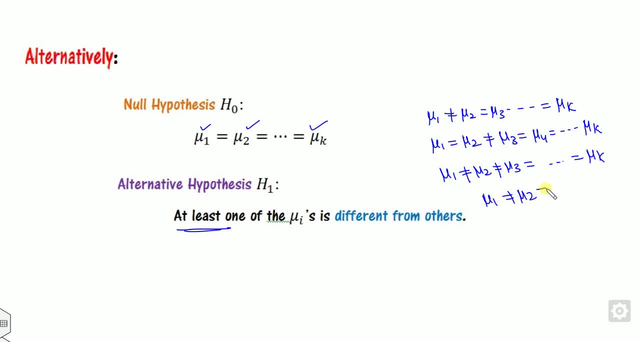 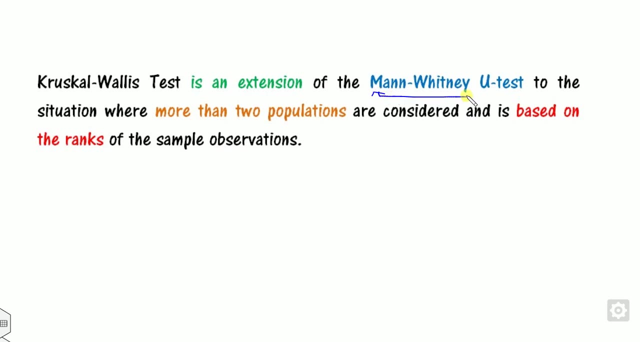 Or you can say: all are not equal. Mu1 is not equal to this is not equal to muK, So any one of them is happening in this alternative hypothesis. Now, what are the extension? is that the crucial wallace is extension of the Mann-Wittner test, And you know that this Mann-Wittner test is used. 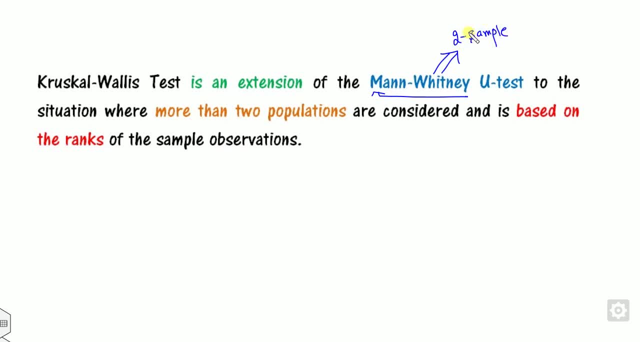 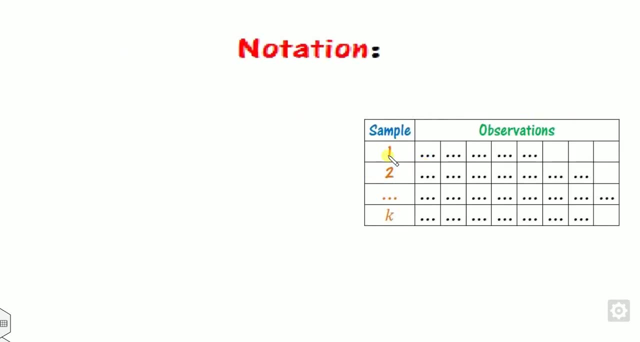 when there is a two sample. So when there is more than two samples, then we will apply the crucial wallace test. So what is the notation, is there? So it must be at least three samples, And these dots are representing my number of the observations. So what I assumption is there are K. samples must be. 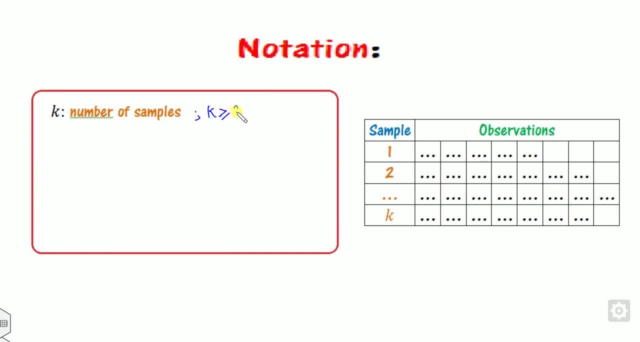 there, And definitely K must be greater than or equal to three. I call as N. i's is the samples, elements in the sample, For example. in this case, how many? What is the N1 is? How many elements are there? Five? What is the N2 is? Look at that. How many? 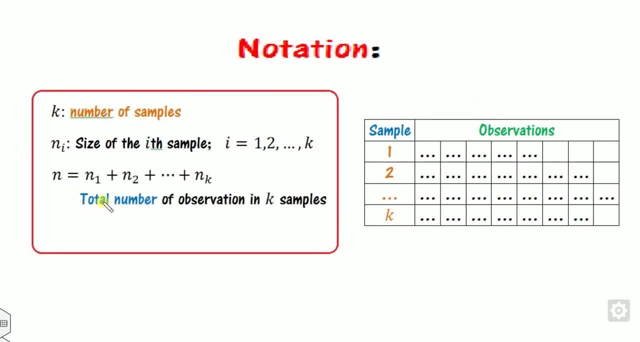 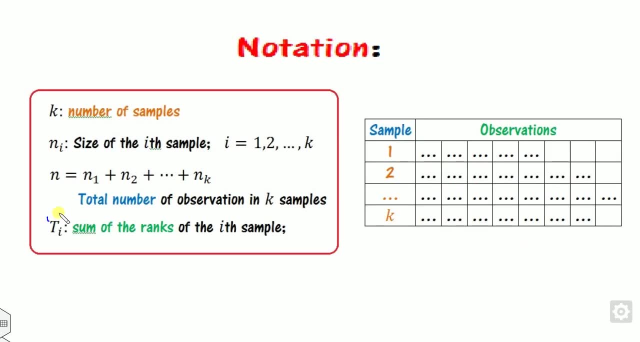 elements are there in seven And so on, And I called as small: n is the total number of the observation. So that is this plus this and so on, And I use the capital T- i is the sum of the ranks. So what is the meaning of the rank? You have to rank the elements, all those elements. 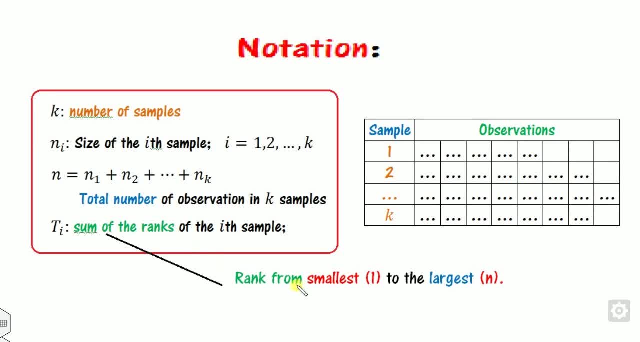 and then find the sum. What is the meaning of the rank is You have to rank from the smallest one to the largest element And if there is any tie between them, you have to take the average. So we will see in the example how we will rank the elements. 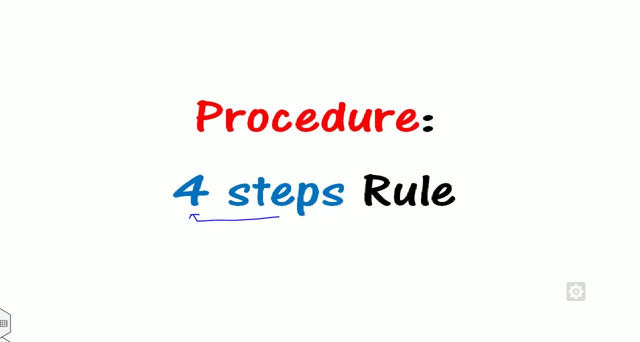 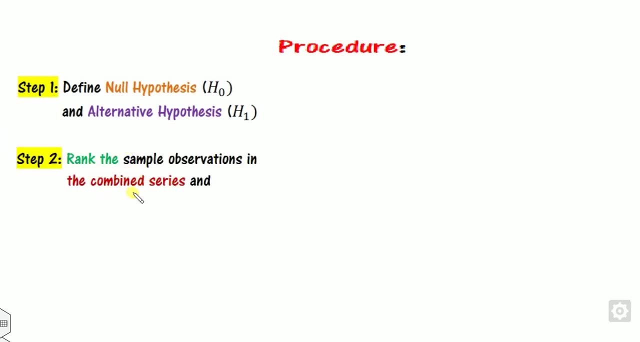 So a simple four-step procedure. we will explain you. First step is you have to define the H0 and H1.. Step two, you have to rank all the observations And once you define all the observation, you have to define the capital T, i sum of the ranks. Once you define. 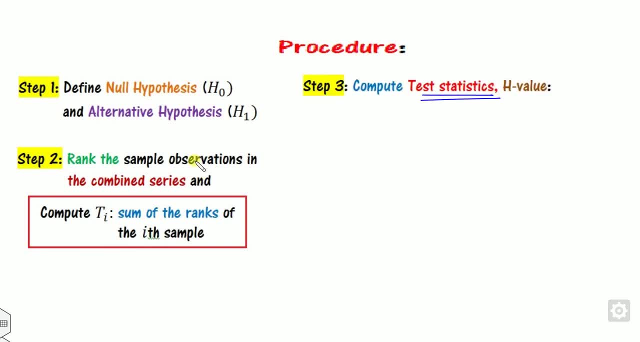 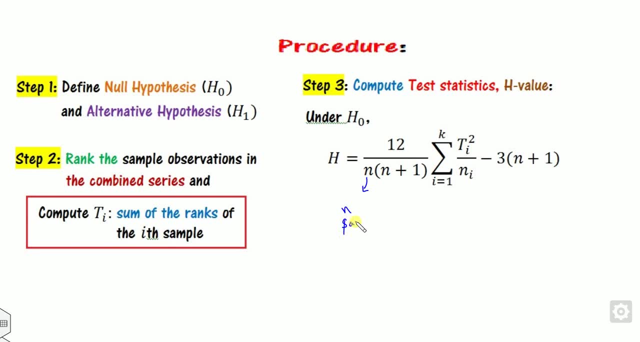 this, then we will define the test statistics, H, which is defined by this way: What is the? n is The sample size. This is the sample size We have calculated how you calculate n is n1 plus n2, and so on. Capital T is my sum of the observation, and so on. Once you calculate this H, 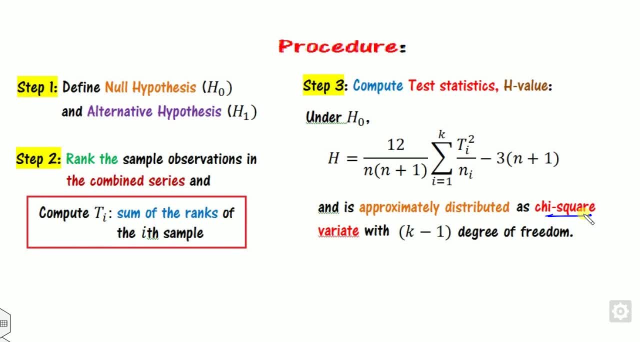 it follows the approximately chi-scale distribution, with the degree of freedom as k minus 1.. What is the k is Number of the samples, So same as that of the one-way ANOVA. We already see that the degree of freedom in the one-way ANOVA is calculated as a k minus 1 also, So you can write: 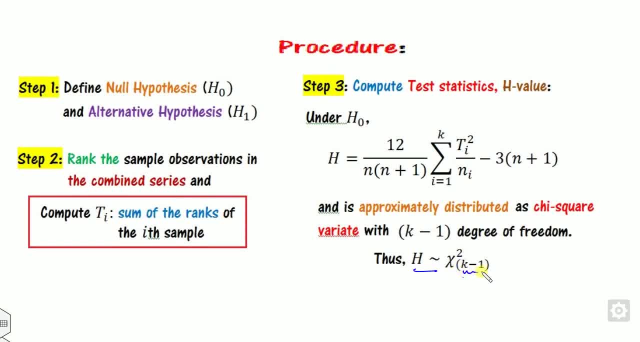 this as H follows chi-scale distribution, with the k minus 1 degree of freedom at alpha level of significance. Once we find this degree of freedom and this value of H, then we will find the tabulated value of the chi-scale. Finally, we will make the decision, as this is 0.. This is the tabulated value and we will check. 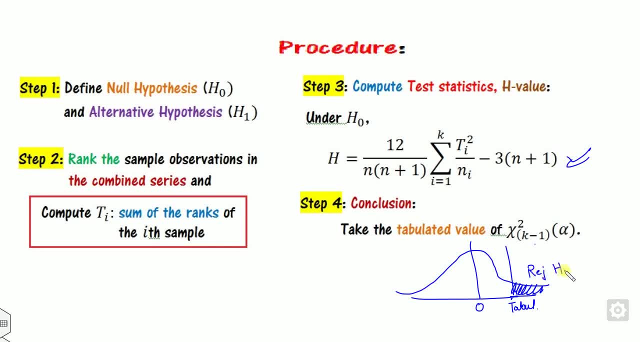 whether this H lies in the rejected H0 or accepted H0.. So look at the example. We will explain you more clearly. So if value of H is greater than of the tabulated value, then we rejected H0. Otherwise, we fail to reject. 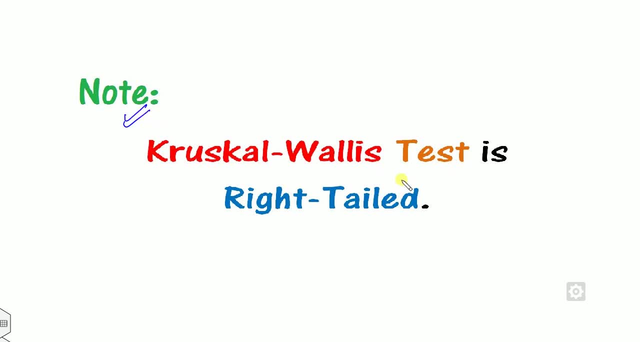 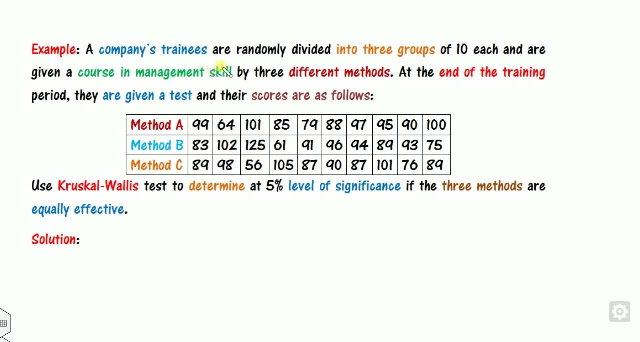 And this is one Most of the most important remark- is it always be the right tail? So look at the example. So a company 20 are randomly divided into three groups. So look at that. There are the three groups. It means the Mann-Whitney test is not applicable, So you have to apply the H test, or 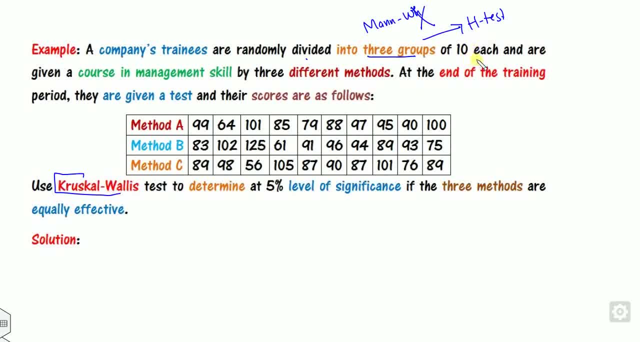 the crucial Wallis test, 10 each, and are given the course of the management skill by the three different methods. So at the end of the trainings the test scores are given here. So what is the? you have to define whether there is any methods are significant or not. So you have to firstly define the H0.. 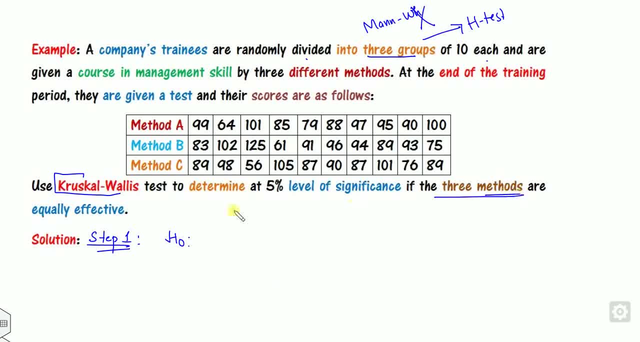 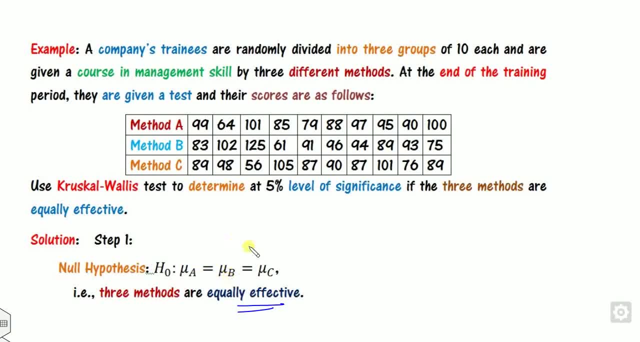 What is the H0? according to the statement, The three methods are equally effective. So what is the H0 is? All the methods are equally effective. Mu A, Mu B, Mu C. What is the H1 is? You can easily. 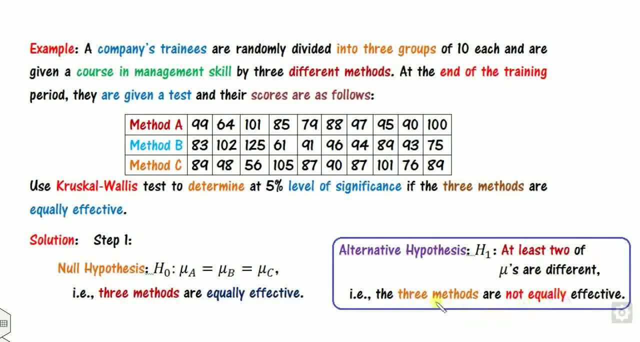 define that At least two of them are Different. or you say: three methods are not equally effective. Now what is the step number two? You have to rank them. How you rank them? There are the several methods are there, So you can rank. 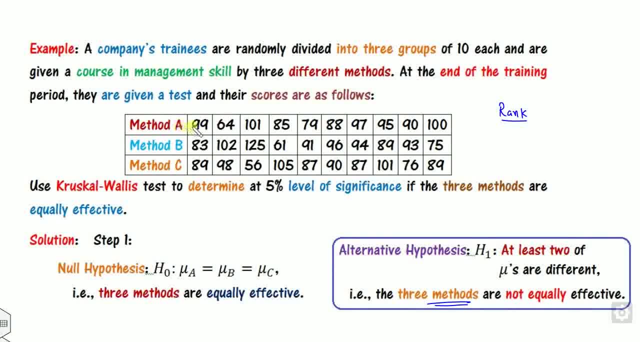 them How you rank. You can rank either the method A- increasing order. method B individually in the increasing order, method C, the value of the method C in the increasing order. Otherwise you can combine them in the increasing order. Look at that. What is the smallest? 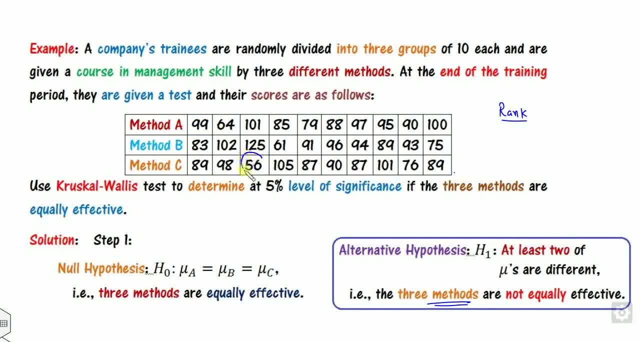 Value in it. Find the smallest value, This 56. So I can write this as the 56.. From which sample it takes C. Look at that. 56 is come from the C And this is the step to compute the rank. 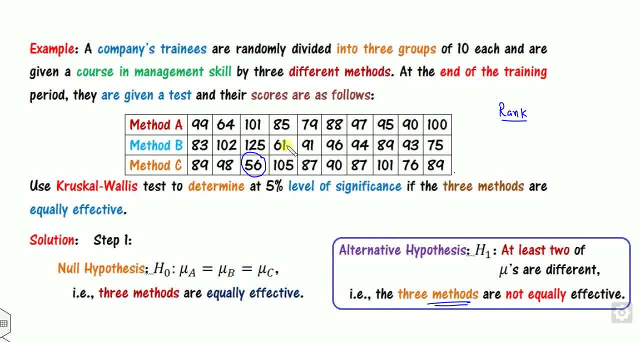 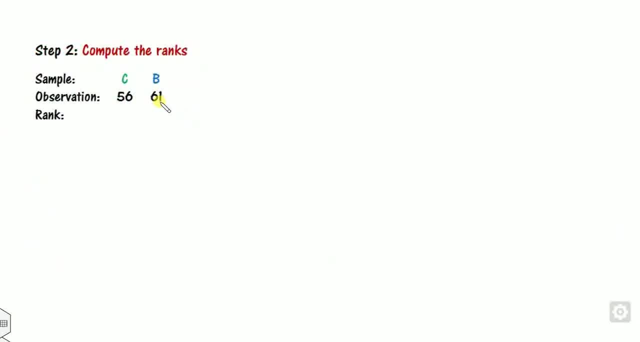 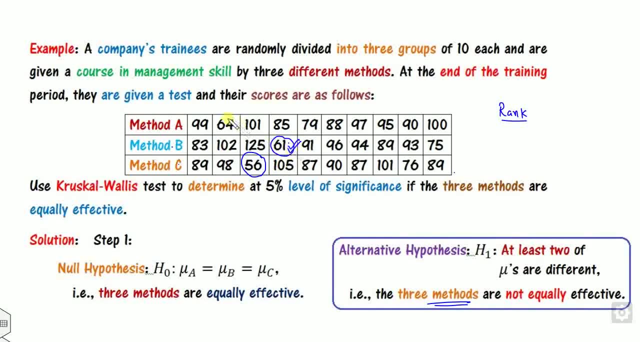 Now look at. the second smallest number is: Can it be 61?? Can it be? Yes, So the next number is 61. So I can write here as 61. It comes from From the B. After that, what is the smallest number is: Is it 64?? Yes, So I can write here. 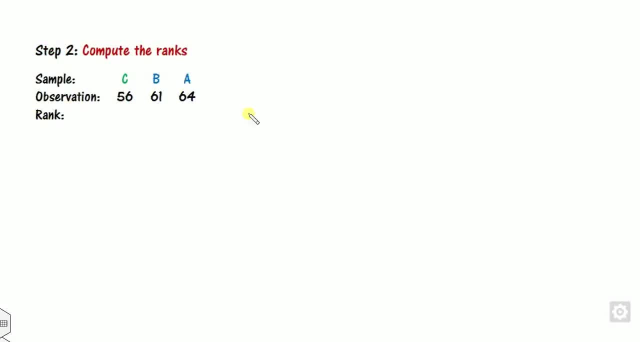 as 64 from the A. Similarly, you can write the: all other values are So this upper are taken from the sample. Now, once you are writing in the ascending order, then you have to take the rank. This is the smallest number. You have to take one. This is the second smallest number. Take two. 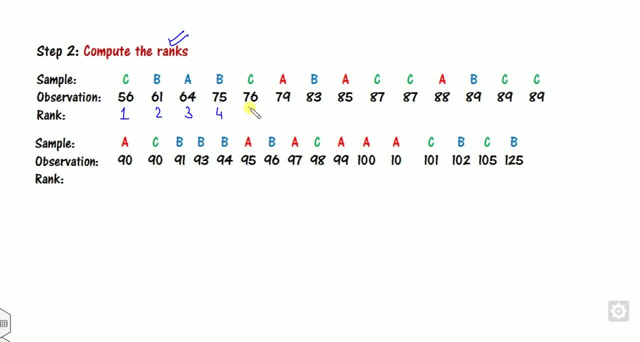 This is the third, This is the, This is the second, Next, This is next, And so on. You will calculate up to here, But after that you can see there is a tie between them. They are the same numbers, So whenever there is a tie. So 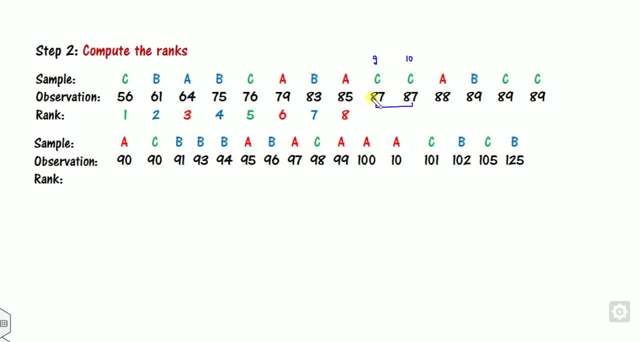 the position of here is 9.. This is a position of 10.. So there are the two numbers. You take the average of them, So it comes to be 9.5.. So here, 9.5, 9.5.. Then now up to here, this is a 10. 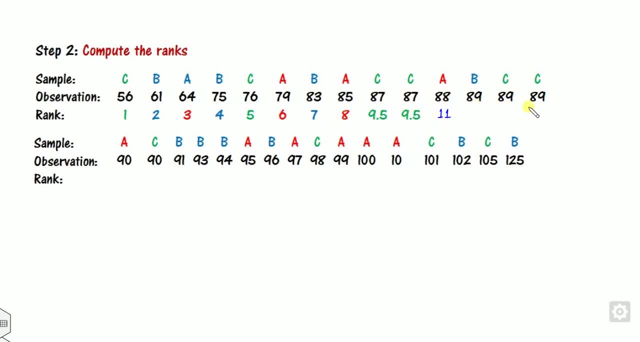 position is there Now, this is 11.. Now there is a tie between them. So how many numbers are there? 12,, 13 and 14.. So there are the three numbers. So take the average of this, Divide it by 3. So it comes to be 13.. So you? 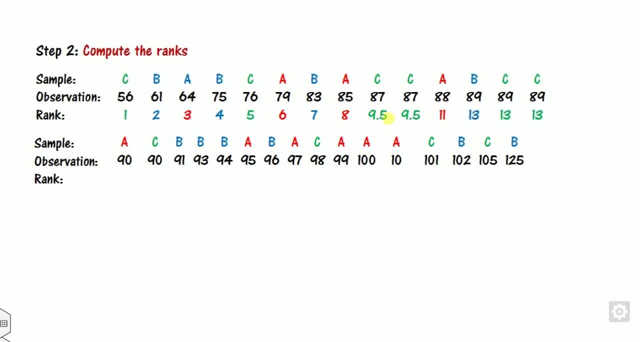 can write here as 13,, 13 and 13.. Now look at for the next number. Now, how many numbers are there? 11,, 12,, 13,, 14.. 12,, 13,, 14.. Now it's come to be 15.. But there are the two repetition, So it's a. 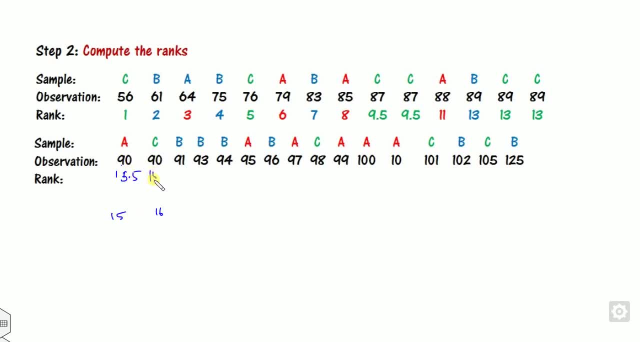 16.. So the repetition is average is 15.5, 15.5 and so on. Now, this is my step, number 2.. Now you can define the n1.. You can define the n2.. You can define the n3.. How many elements in the a? 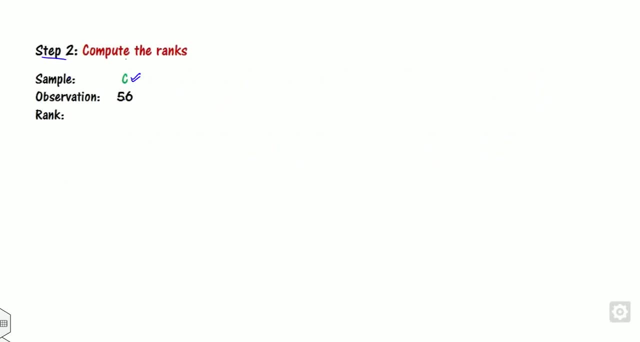 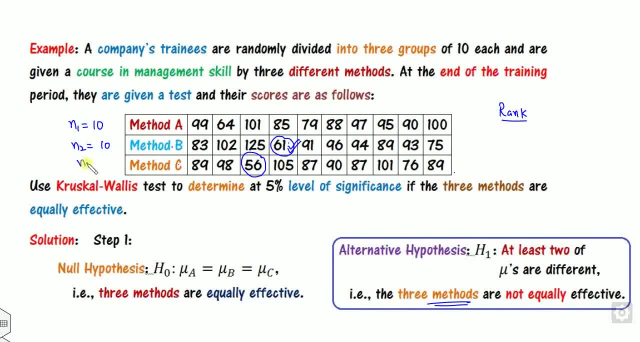 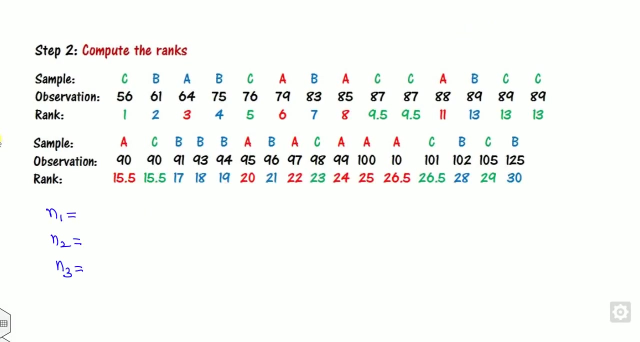 You can take it from this. simply Look at the given observation. How many elements in the a is 10.. How many elements in the b is again 10? How many elements in the c Is again 10.. So you can write here as my n1,, n2 and n3 as this: So what is the n is Total of. 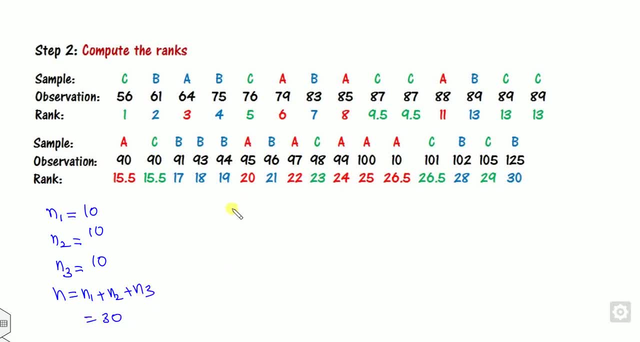 them. So it is 30.. Now you define the t1.. What is the t1 is Sum of the ranks of the first sample. First sample is my a. So what are the elements of the a? These are the. 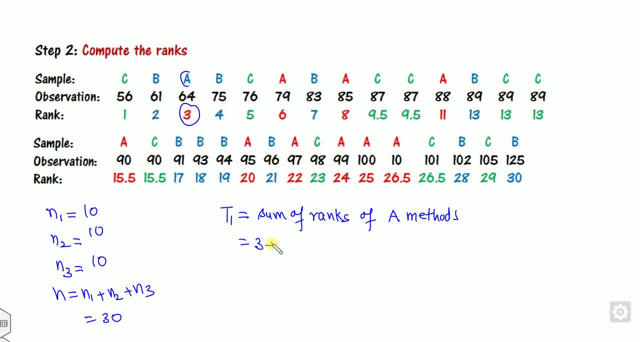 elements of a. So rank is 3.. So what is the t1 is 3. Plus what are the rank of a 6. a is 8., a is 11., a is 15.5. Plus a is my 20.. Next, a is 22.. 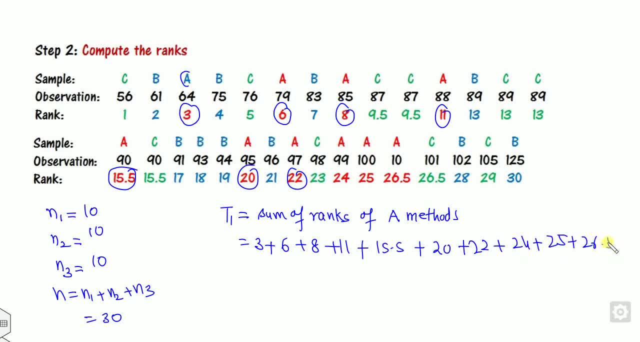 Then 24, 25 and 26.5.. This is my t1. Similarly you can find the t2.. Sum of the ranks of the b methods c and c. This is the first sample. Now you can define the n1.. How many elements in the? 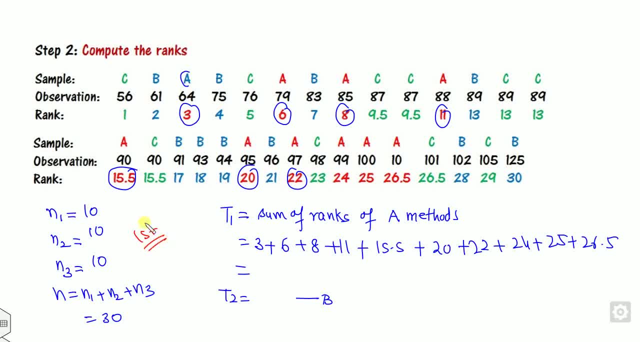 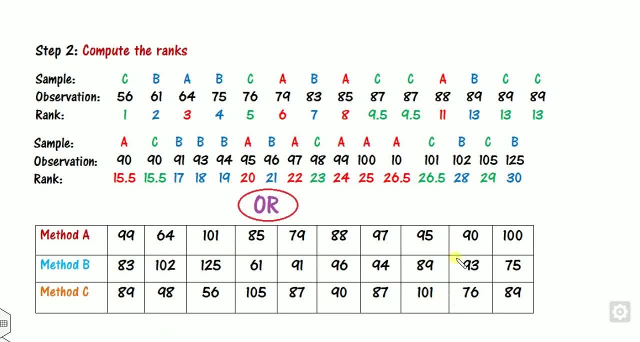 c Is green and yellow. This is my a. So another method is Ans, which is green and yellow. Where A means Press you, A is h or h is a And B means Graph, C means That numbers stand off, or A is ae and B means Every follows. 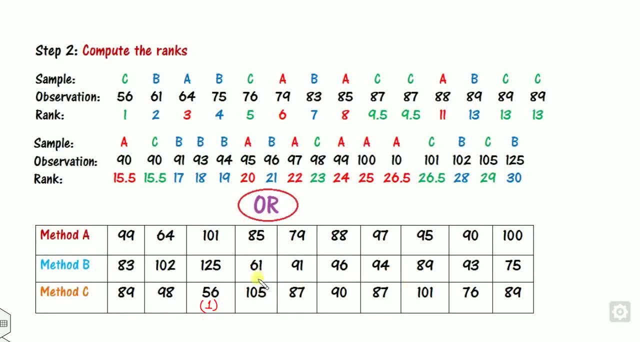 the same order is negative. So if the number is negative, choose other numbers in which you can find the value of A and N. Where is b? where is g? c? bur g is advent, A is in between two, C is in between two, A is in between zero expression and A is tuck. 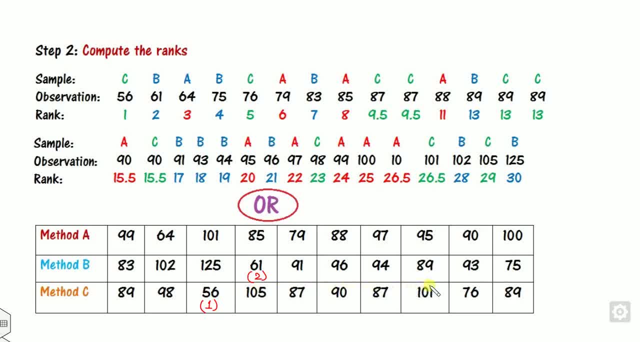 C is in between zero expression and A is in between two. All right. The second important part is the a Same thing as a if number is notiche number, for example q, c, a, h, b. what is the next smallest number is 64. place the rank number 3 instead of. 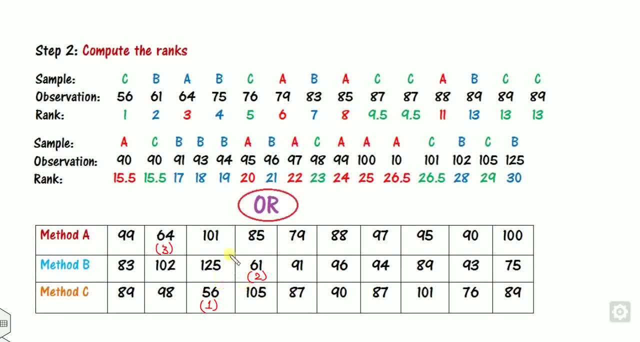 writing in the ascending, descending. you can write directly from here. what is the next smallest number is 75. take the rank as a 4. next smallest number is 76. take the rank as a 5. next one is: what is the smallest number is 79. is a 6 then is my. 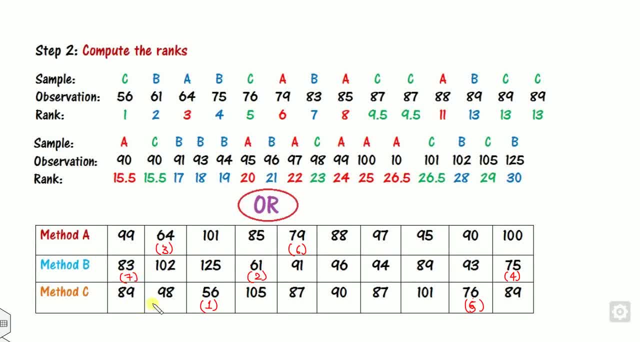 83, 7. then the smallest number is 87. no, it's 85, it's 8. now there is a tie between the 87 and 87, so 9 and 10. so take the average, it's a 9.5. it's a 9.5. 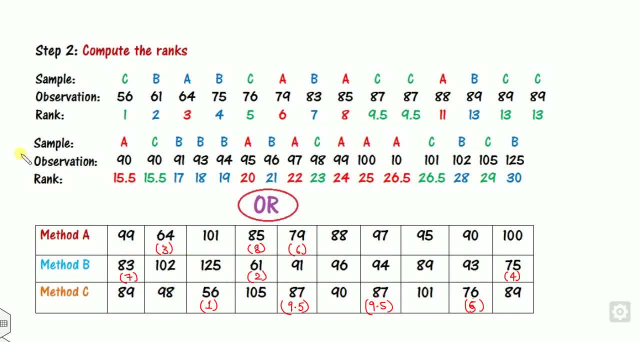 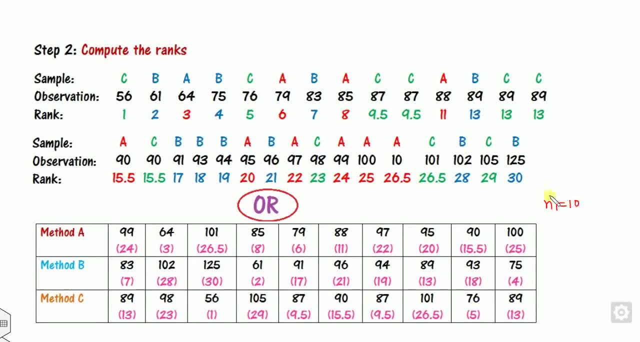 and so on. so once you will complete all those entries, you will get this one. okay, then how you find the end when n 1 is remain same, 10 and 2 is my 10. look at that and then you will get the result of that. you will get the result of that. 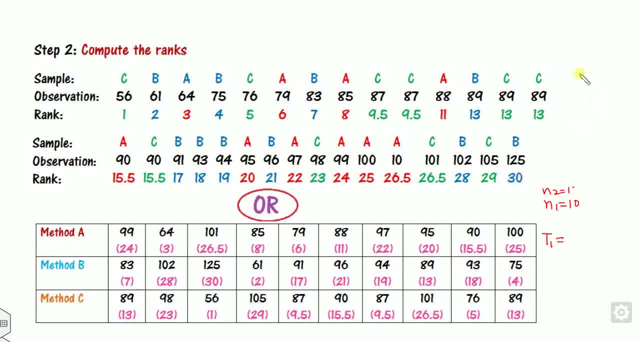 and then you will get the result of that, and then you will get the result of that. that 10 elements- so how you define the t1 is in this method. you have to look at. that 10 elements- so how you define the t1 is in this method, you have to look at. 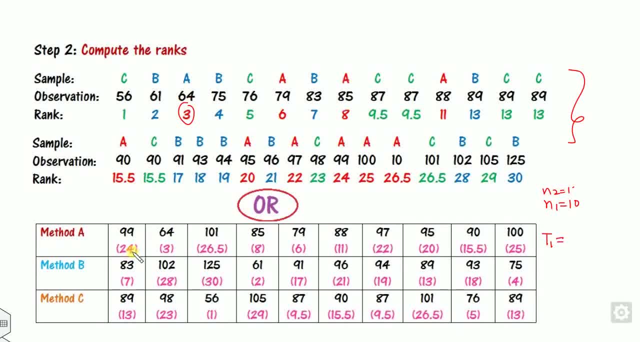 for the a and so on. in this case you have to add them 24 plus 3 plus this for the a and so on. in this case you have to add them 24 plus 3, plus this, plus this, plus this up to 25 is my t1. how you find that t2? that is a rank of. 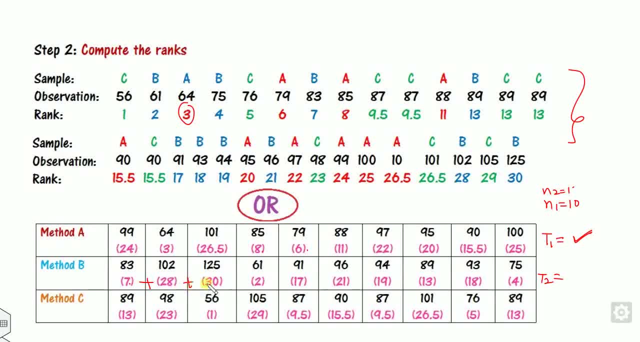 plus this up to 25, is my t1. how you find that t2- that is a rank of. the second is the 7 plus 28 plus 30 plus 2 plus 17 plus 21, and so on. this is my. the second is the 7 plus 28 plus 30 plus 2 plus 17 plus 21, and so on. this is my. 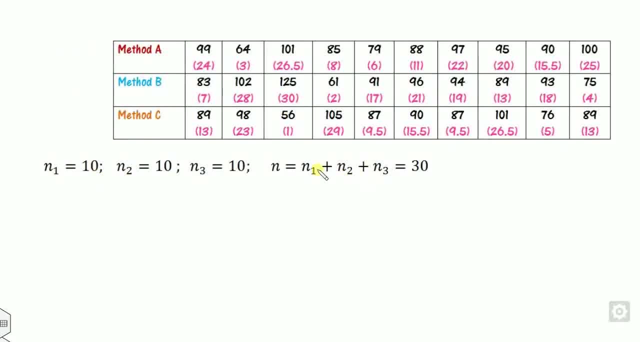 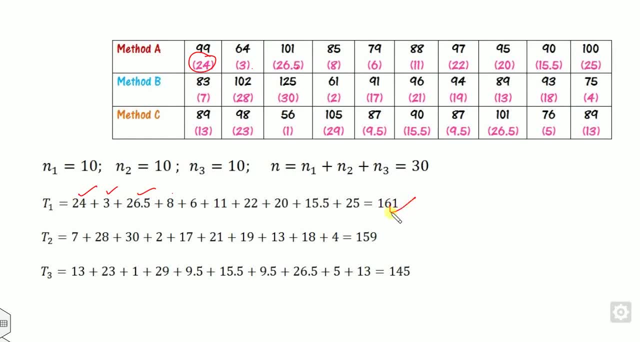 t2 and so on. so look at that. these are there, how you define the t1. look at that. these are there. how you define the t1. look at that. these are there. how you define the t1 from this, from this, from this. look at that: 24, 3 plus 26.5 and so on. so 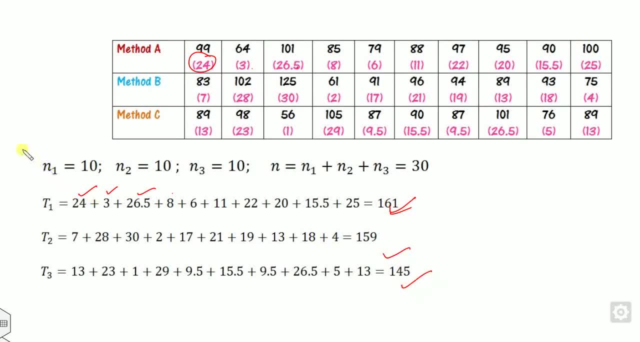 look at that: 24, 3 plus 26.5, and so on. so look at that: 24, 3 plus 26.5, and so on. so this is my t1, t2 and t3. this is my t1, t2 and t3. 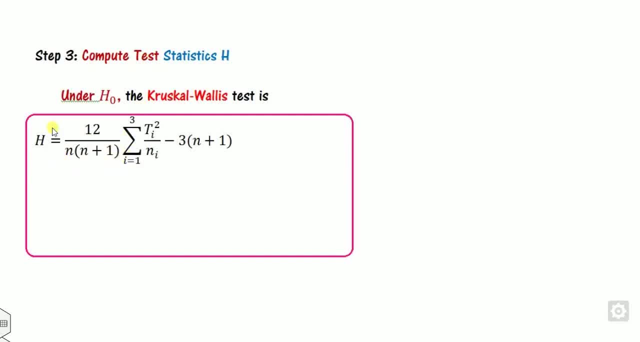 this is my t1, t2 and t3. now step third is you have to define this now. step third is you have to define this now. step third is you have to define this. what is the n? is n? is my 30 t1? is this 3? what is the n? is n is my 30 t1, is this 3? what is the n? is n is my 30 t1, is this 3? and so on. you can substitute the value, and so on. you can substitute the value, and so on. you can substitute the value here. 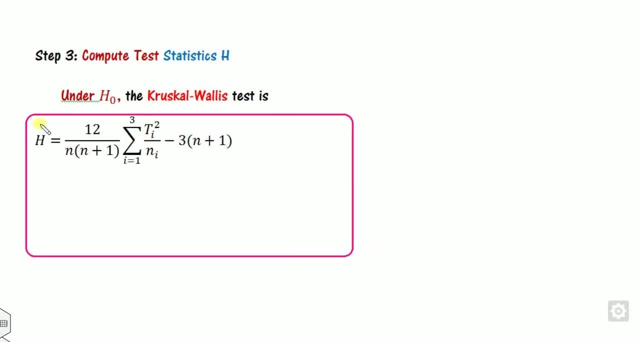 here: 12 divided by this: what is the t1? look at 12 divided by this: what is the t1? look at 12 divided by this: what is the t1? look at that: that t1 is my 161 and 1 is my 10. 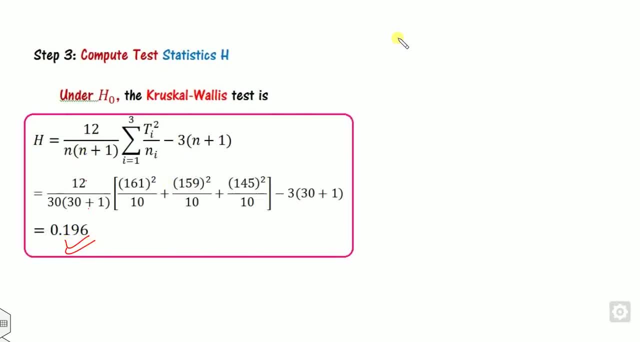 that that t1 is my 161 and 1 is my 10, that that t1 is my 161 and 1 is my 10. so you can calculate this here. so you can calculate this here. so you can calculate this here. now, step number four: 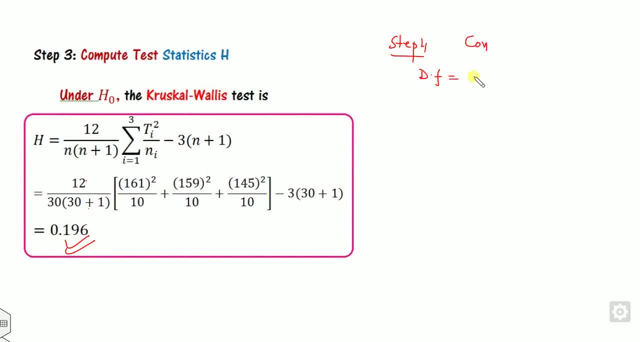 now step number four. now step number four. that's the conclusion you have to find. that's the conclusion you have to find, that's the conclusion. you have to find the degree of freedom, the degree of freedom, the degree of freedom k minus one. how many samples are there? 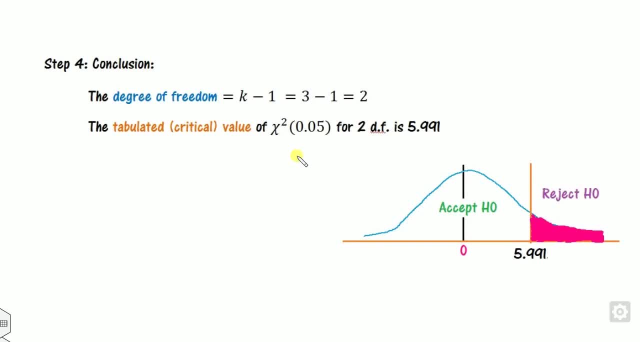 k minus one. how many samples are there? k minus one. how many samples are there? three. so degree of freedom is my three. so degree of freedom is my three. so degree of freedom is my two, two, two. given level of significance for the two. given level of significance for the two. 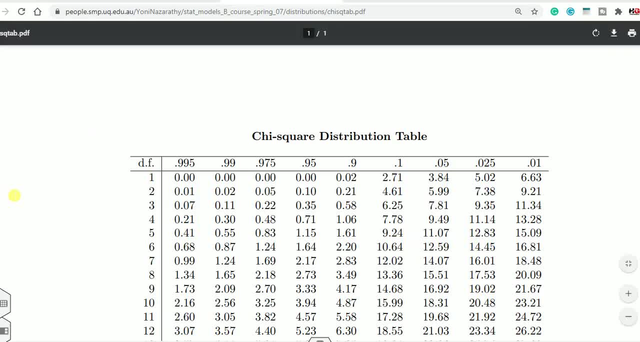 given level of significance for the two tail. how you find this value. so look at tail. how you find this value. so look at tail. how you find this value. so look at that this is a chi-square distribution, that this is a chi-square distribution, that this is a chi-square distribution table. how you find that. you can write on. 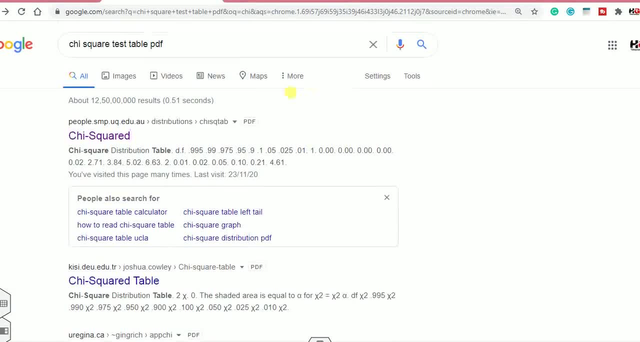 table. how you find that you can write on table. how you find that you can write on the google as a chi-square table. you can the google as a chi-square table. you can the google as a chi-square table. you can simply write the chi-square t-test table. 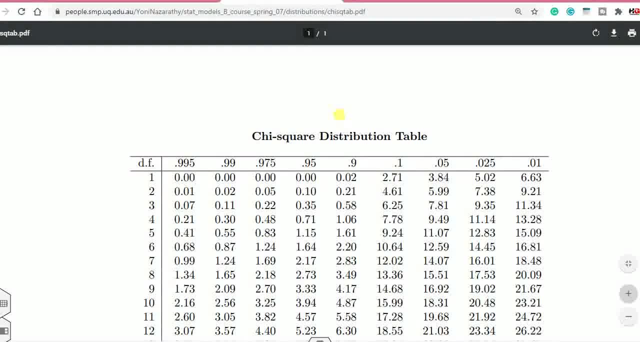 simply write the chi-square t-test table. simply write the chi-square t-test table. the first link will appear. you can open. the first link will appear. you can open. the first link will appear. you can open them. then look at the. what is the degree them. then look at the what is the degree. 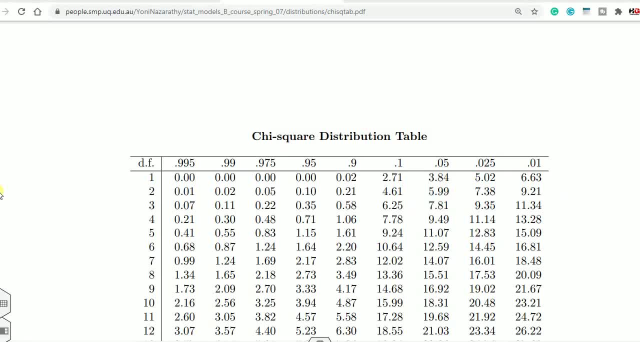 them. then look at the. what is the degree of freedom? is two of freedom is two of freedom is two. and look at that degree of freedom is two. and look at that degree of freedom is two. and look at that degree of freedom is two here, here, here, and the level of significance is 0.05. so 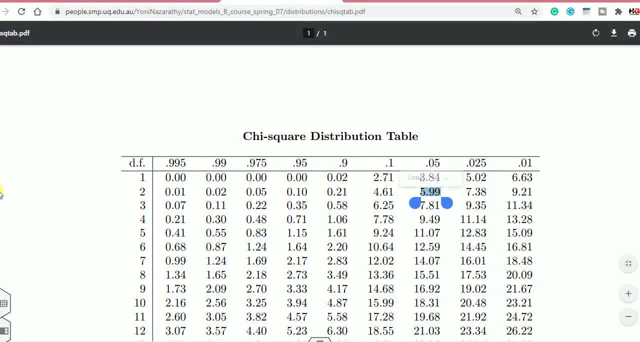 and the level of significance is 0.05. so, and the level of significance is 0.05, so what is the value is what is the value is? what is the value is 5.91. you can see that. so this is the 5.91. you can see that, so this is the. 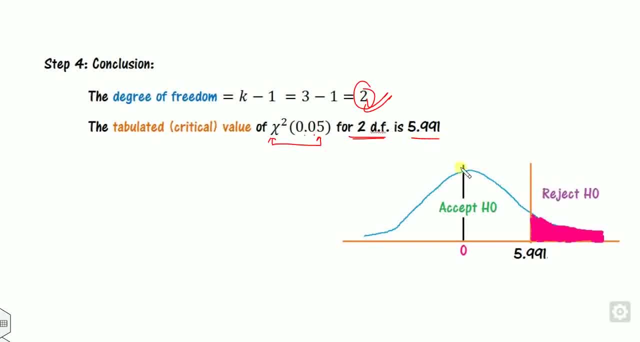 5.91. you can see that. so this is the tabulated value of the 5.91 here. tabulated value of the 5.91 here. tabulated value of the 5.91 here. so this is the you can write up to two. 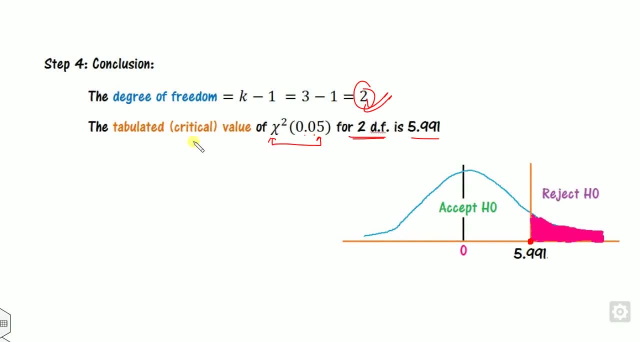 so this is the you can write up to two. so this is the. you can write up to two, or up to the three decimal places, or up to the three decimal places, or up to the three decimal places. now, what is the calculated value of the? now, what is the calculated value of the? 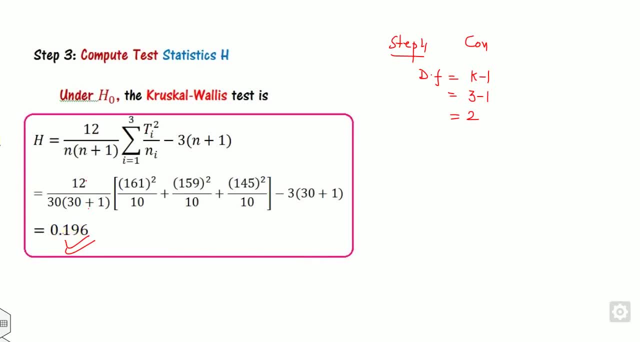 now, what is the calculated value of the chi point h 0.196? chi point h 0.196. chi point h 0.196: where it lies? it lies here because it where it lies. it lies here because it where it lies. it lies here because it lies between zero, so it is. 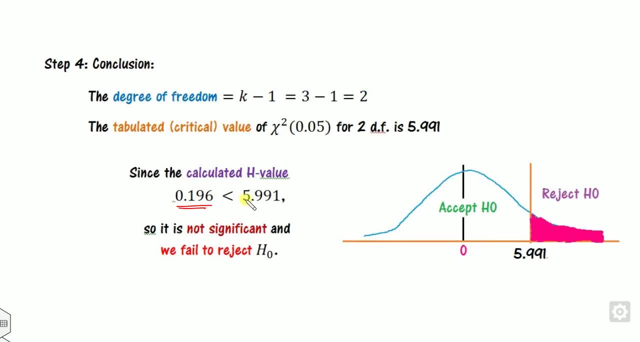 lies between zero, so it is lies between zero, so it is maybe accepted. so, since the calculated maybe accepted, so since the calculated maybe accepted, so since the calculated value is value is value is less than of this, so we fail to less than of this, so we fail to. 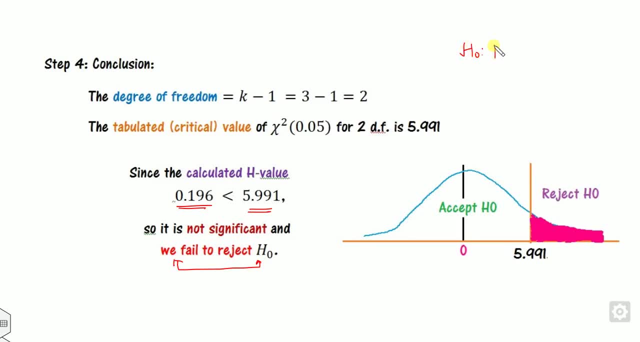 less than of this. so we fail to reject h0. what is your h0? reject h0. what is your h0? reject h0. what is your h0? that is: this was your h0. that is, this was your h0. that is, this was your h0. that is all the teaching methods are. 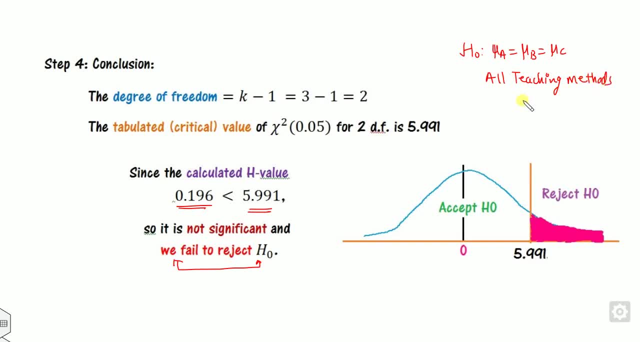 that is, all the teaching methods are. that is, all the teaching methods are equal, equal, equal. all the teaching methods are equal. all the teaching methods are equal. all the teaching methods are equal. this is your h0 and it is accepted. this is your h0 and it is accepted. 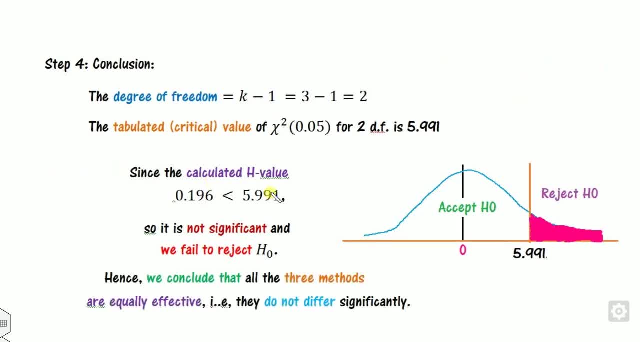 this is your h0 and it is accepted. so what you conclude that you can say. so what you conclude that you can say. so what you conclude that you can say: the t, all the methods are do not differ. the t, all the methods are do not differ. 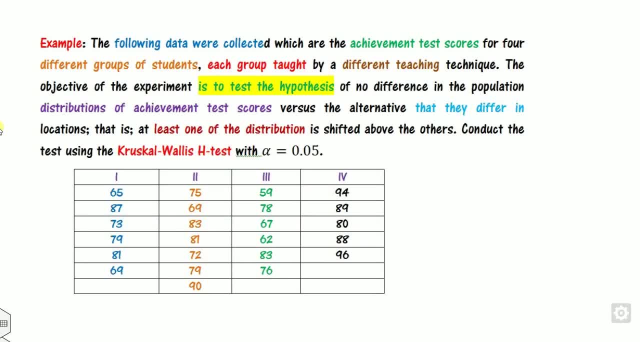 the t all the methods are do not differ significantly, significantly, significantly. now let's do quickly move example second. now let's do quickly move example second. now let's do quickly move example second, so it will clear more, so it will clear more, so it will clear more to you. so these are some tests are there. 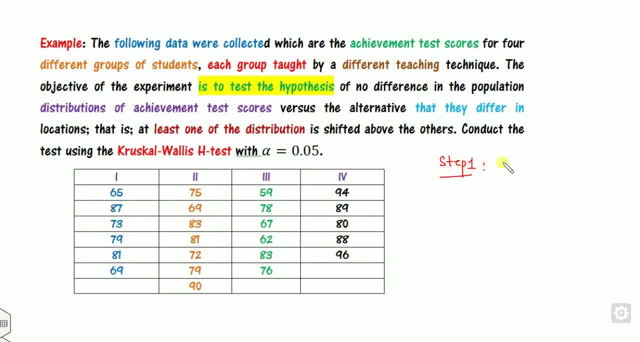 to you. so these are some tests are there to you. so these are some tests are there, so. so, so, how you define that you have to start, how you define that you have to start, how you define that you have to start with a step, with a step. 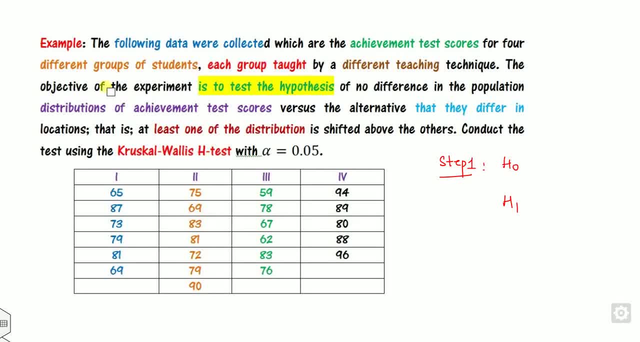 with a step one: h0 and h1. so look at that. what is your one? h0 and h1. so look at that. what is your one? h0 and h1? so look at that. what is your h0? so h0, so h0. so the objective of the experiment is to test. 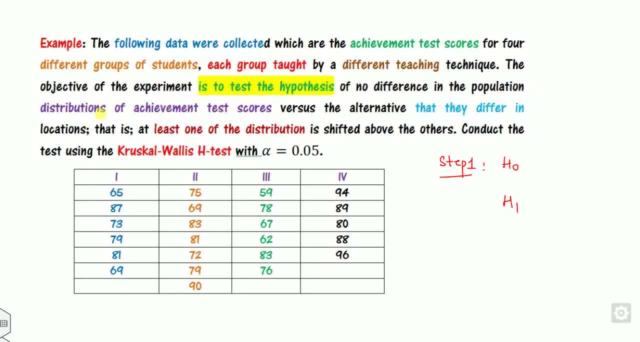 the objective of the experiment is to test. the objective of the experiment is to test the hypothesis of the hypothesis, of the hypothesis of no difference in the population. no difference in the population, no difference in the population. distribution versus, distribution versus, distribution versus. there is a difference in the population. so 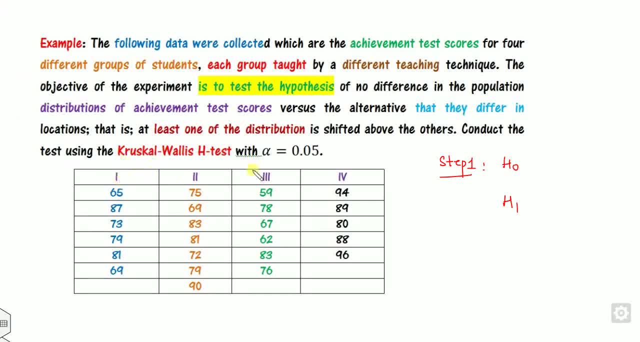 there is a difference in the population. so there is a difference in the population. so what is the h0? what is the h0? what is the h0? that there are the four samples, that there are the four samples, that there are the four samples and each sample consists of more than. 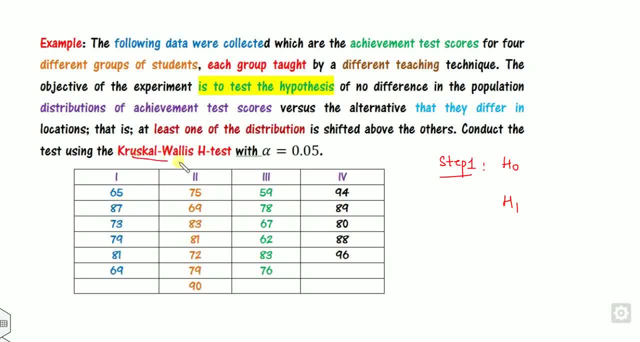 and each sample consists of more than. and each sample consists of more than five elements. five elements, five elements or five elements. so the crucial wallace or five elements. so the crucial wallace or five elements. so the crucial wallace. test is applicable. test is applicable. test is applicable. so what is that? this? you can say all the 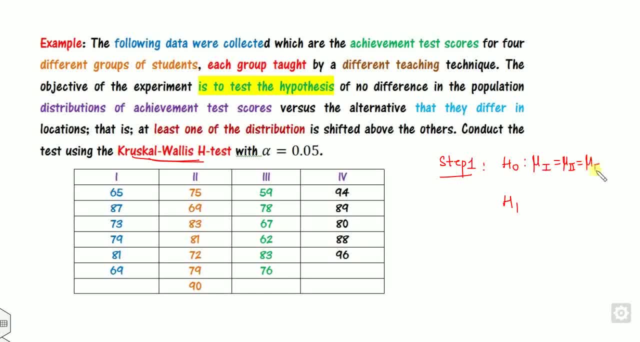 so what is that this? you can say: all the. so what is that this? you can say: all the four samples are equal: mu1, mu2, mu3 and mu4, and here is at least one of them differ. and here is at least one of them differ. 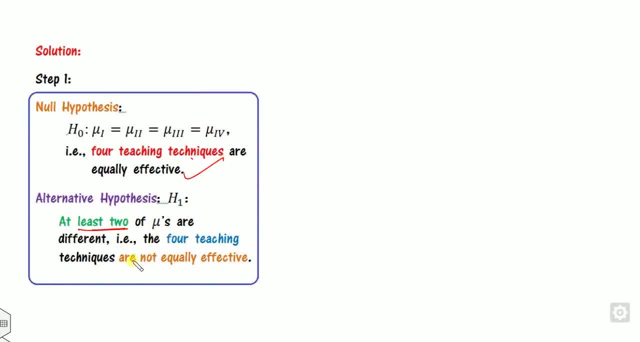 and here is at least one of them differ. all the four teaching are equal, or at all the four teaching are equal, or at all the four teaching are equal, or at least two of them, least two of them, least two of them differ. what is the step two is you have to. 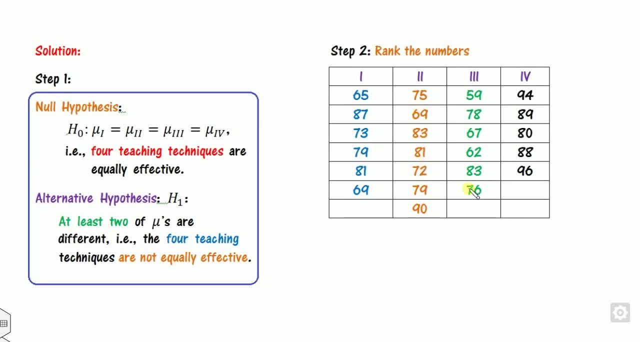 differ. what is the step two? is you have to differ. what is the step two is you have to rank the elements, rank the elements, rank the elements. so these are the given observation. so so, these are the given observation. so so, these are the given observation. so the one method is you can write in the 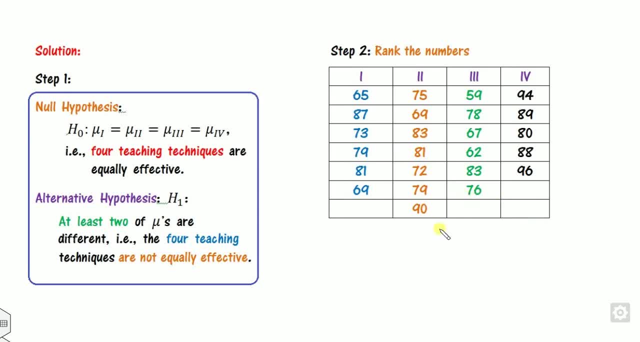 the one method is you can write in the. the one method is you can write in the increasing or descending order. increasing or descending order, increasing or descending order, but there is no need of them. you can, but there is no need of them. you can, but there is no need of them. you can write here: what is the smallest number in. 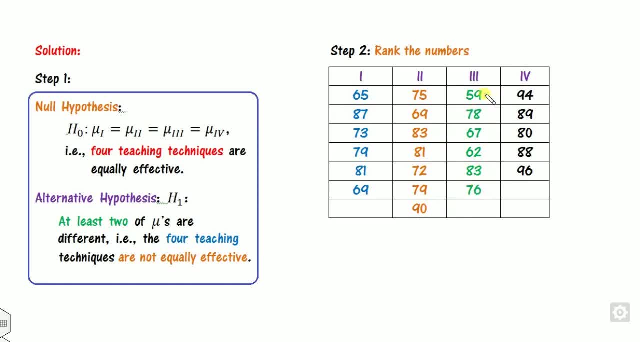 write here. what is the smallest number in write here. what is the smallest number in in this here. look at the. what is the in this here? look at the. what is the in this here. look at the. what is the smallest number is smallest number is smallest number is 59. you can rank them as a one. 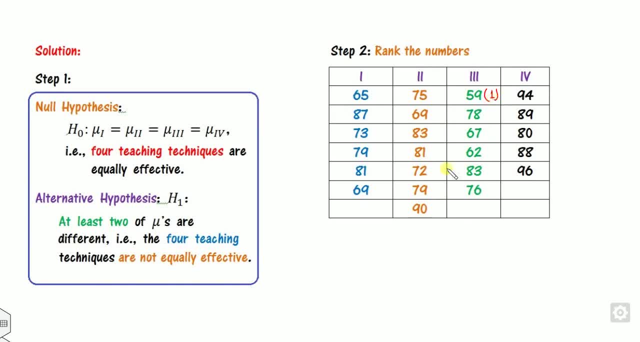 59. you can rank them as a one. 59, you can rank them as a one. look at the next smallest number in them. look at the next smallest number in them. look at the next smallest number in them is: is: is this 59 is 62? put them as a number two. 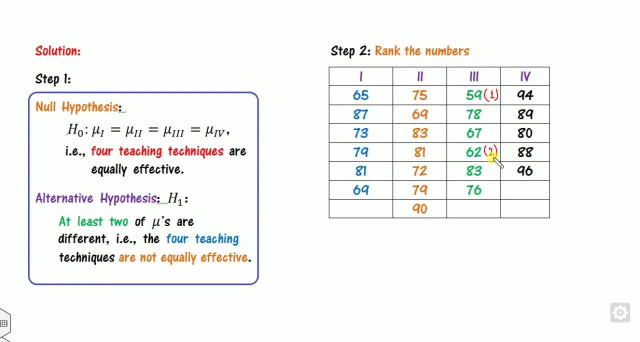 this 59 is 62. put them as a number two. this 59 is 62. put them as a number two. what is the next smallest number inside? what is the next smallest number inside? what is the next smallest number inside? it is, it is. it is 69. it appears one here. it appears one. 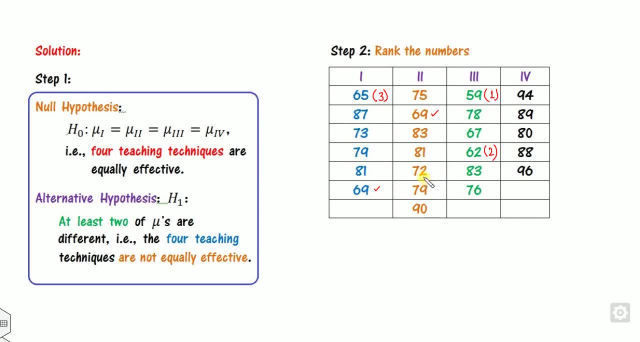 69. it appears one here. it appears one: 69, it appears one here. it appears one more time. so it's appeared two times more time. so it's appeared two times more time, so it's appeared two times. it's appears two times, as here, so look. 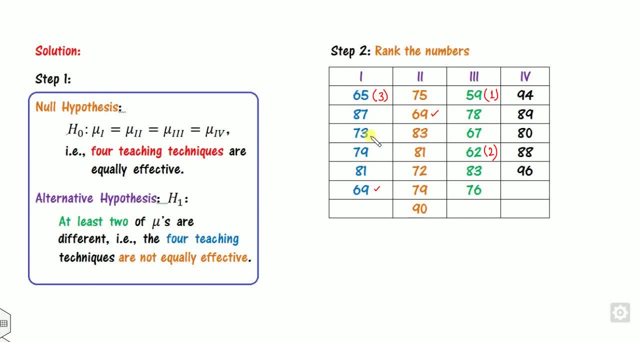 it's appears two times, as here. so look, it's appears two times as here. so look at that. one, two, three at that. one, two, three at that. one, two, three. what is that? so it's a no, it's a 67. what is that? so it's a no, it's a 67. 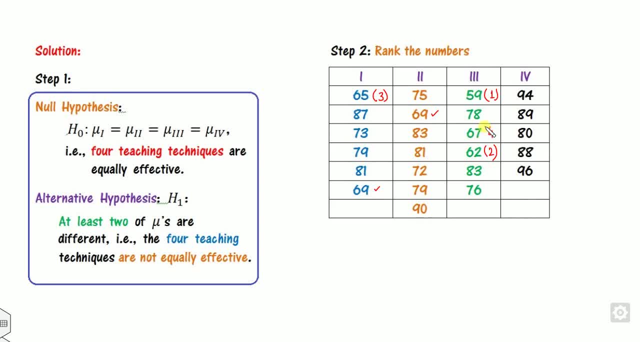 what is that? so it's a. no, it's a 67 also, also, also so, firstly, it's one time only. so it's a. so, firstly, it's one time only. so it's a. so, firstly, it's one time only. so it's a four, four. 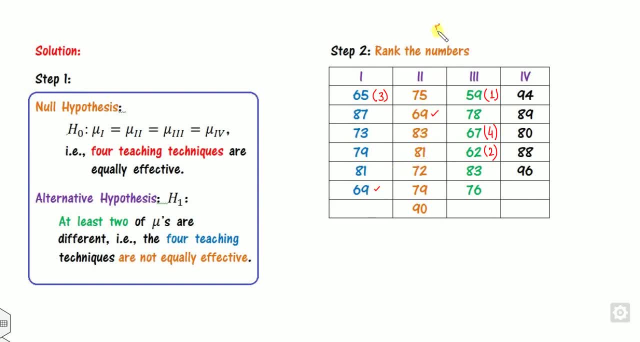 four, now 69. it appears two times the position, now 69. it appears two times the position- now 69. it appears two times the position is five and six. so take the average is five and six. so take the average is five and six. so take the average: 5.5 here and 5.5 here. 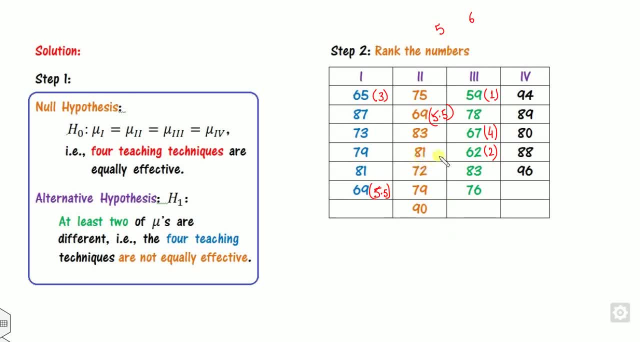 then now six opposition are there. what then now six opposition are there. what then now six opposition are there? what is this next number is? is this next number is: is this next number is now seven. seventh number is there, so now seven. seventh number is there, so now seven. seventh number is there. so look at that. the smallest number is 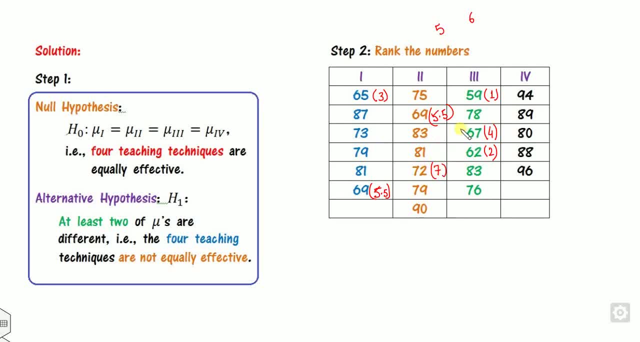 look at that, the smallest number is. look at that: the smallest number is 72, 72, 72. so it's a seven, so it's a seven, so it's a seven, and so on. okay, so, once you will do that, and so on. okay, so, once you will do that. 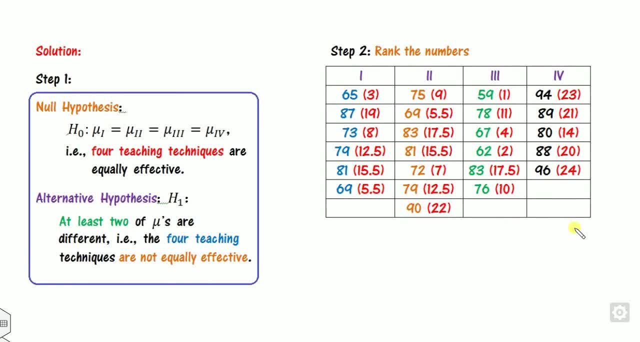 and so on. okay, so once you will do that, you can find all these ranks are here. you can find all these ranks are here. you can find all these ranks are here now, once you are finding all the ranks, now, once you are finding all the ranks now, once you are finding all the ranks, look at that. what is the n1? how many? 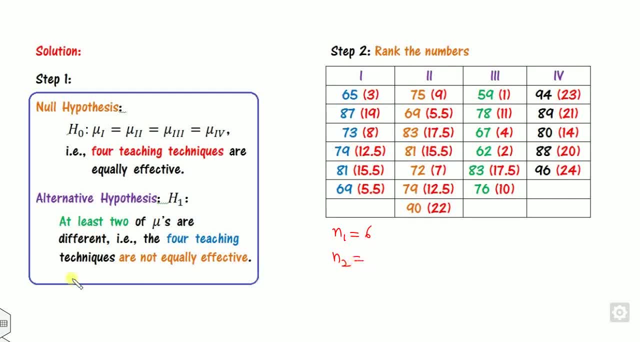 look at that. what is the n1? how many? look at that. what is the n1? how many elements are there? elements are there. elements are there six. what is the n2? how many elements are six? what is the n2? how many elements are six? what is the n2? how many elements are there is? 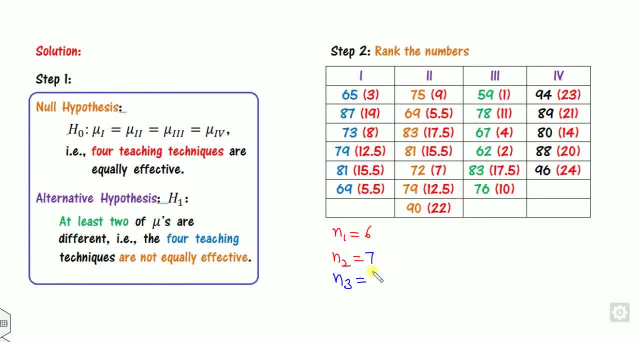 there is. there is seven. what is the entries? how many? seven? what is the entries? how many? seven? what is the entries? how many elements are there? elements are there. elements are there. it's a six. what is the n4? how many? it's a six. what is the n4? how many? 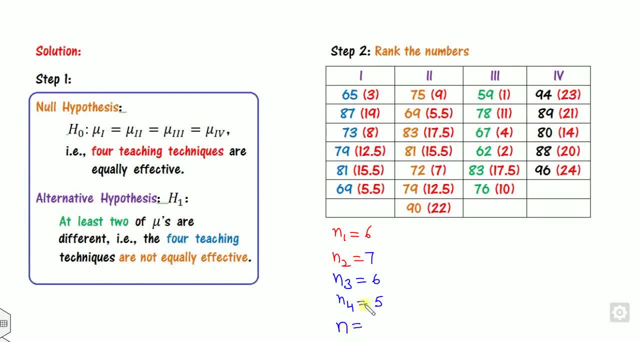 it's a six. what is the n4? how many elements are there? elements are there. elements are there five. so what is the n? that is a total five. so what is the n? that is a total five. so what is the n? that is a total. okay, so that is my 24.. 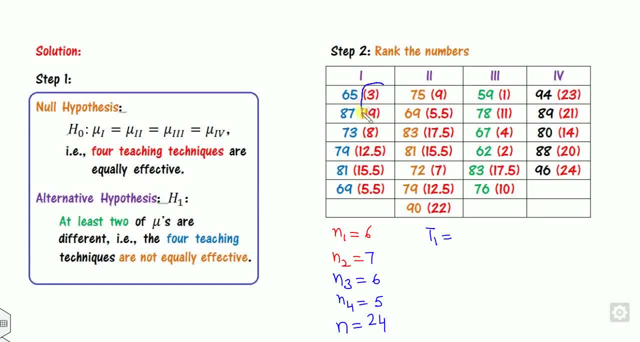 okay, so that is my 24.. okay, so that is my 24.. what is that t1? what is that t1? what is that t1? sum of this ranks. these are the ranks. sum of this ranks. these are the ranks. sum of this ranks. these are the ranks. so how you define 3 plus 19 plus. 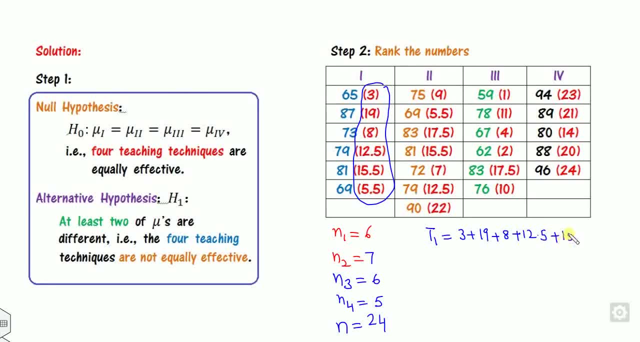 so how you define 3 plus 19 plus. so how you define 3 plus 19 plus 8 plus 12.5, 8 plus 12.5, 8 plus 12.5 plus 15.5 plus 5.5. 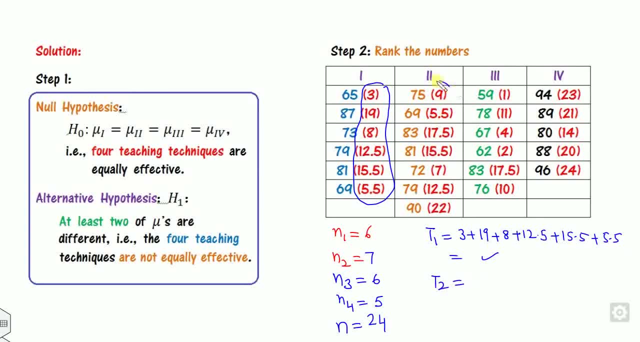 plus 15.5 plus 5.5 plus 15.5 plus 5.5, so you can get t1. similarly for the t2. so you can get t1. similarly for the t2, so you can get t1. similarly for the t2. you can add these elements: 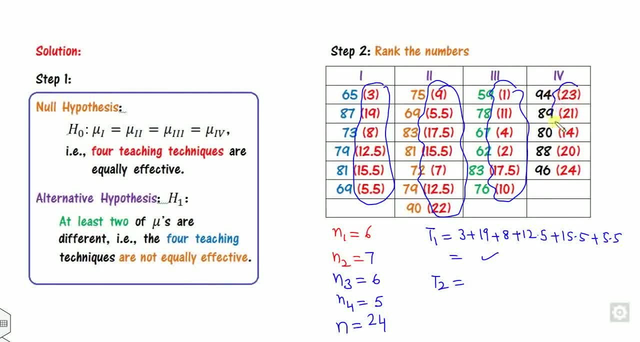 you can add these elements. you can add these elements similarly for the t3. you can find this similarly for the t3. you can find this similarly for the t3. you can find this: ranks and these are the x. so this is ranks and these are the x. so this is. 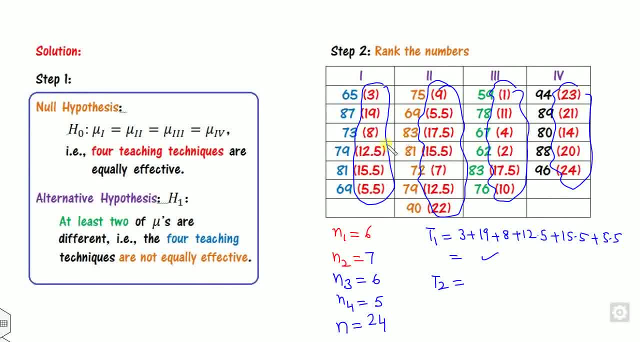 ranks and these are the x. so this is quite easy way you can rank. add them, quite easy way you can rank. add them quite easy way you can rank. add them here instead of writing all in the here, instead of writing all in the here, instead of writing all in the ascending or descending order. so once 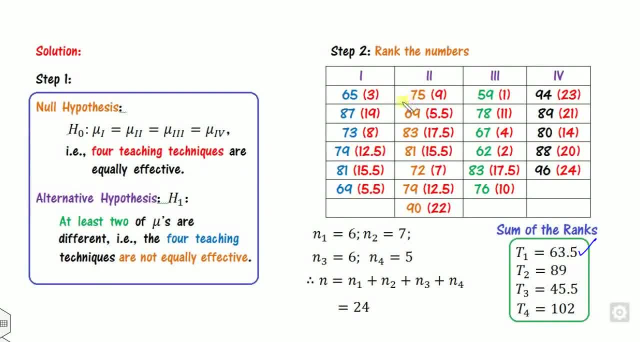 ascending or descending order. so once ascending or descending order, so once you will add them, you will get. you will add them, you will get, you will add them. you will get 63.5 as the sum of this, 63.5 as the sum of this. 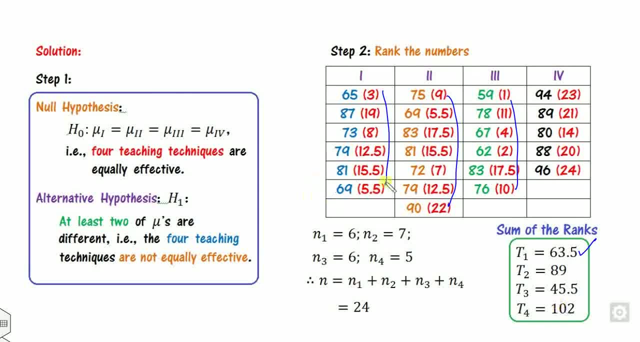 63.5 as the sum of this: 89 is here, this and this now. this is 89 is here. this and this now. this is 89 is here. this and this now. this is step 2. step 33 is you have to calculate? step 2, step 33 is you have to calculate? 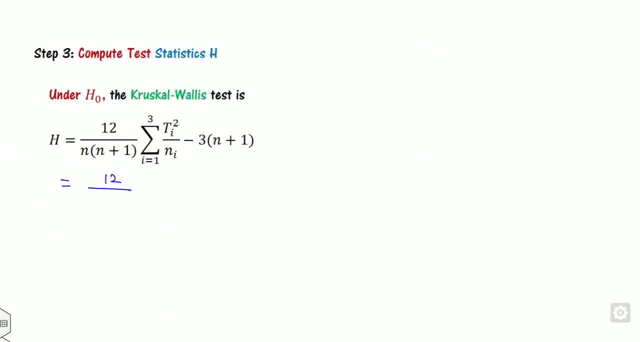 step 2. step 33 is: you have to calculate the value of z, the value of z, the value of z. now you can substitute here what is the n. now you can substitute here what is the n. now you can substitute here what is the n is. 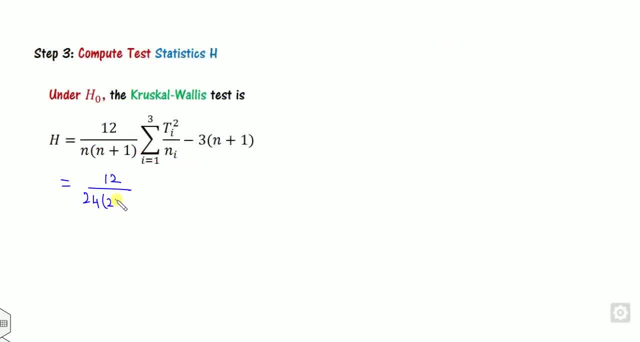 is is 24, so it is my 24, and 24 plus 125: 24, so it is my 24 and 24 plus 125 24, so it is my 24 and 24 plus 125. what is that t1? what is that t1? 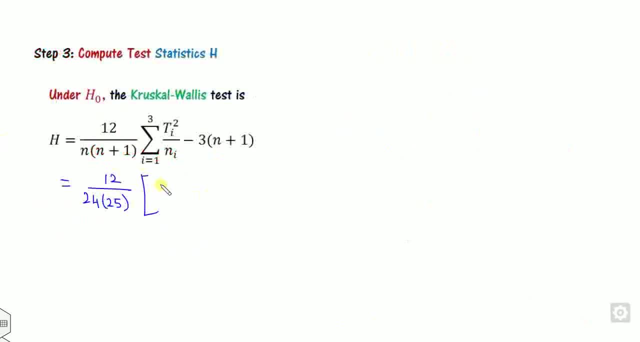 what is that? t1: 63.5 and n1 is my six. so this is my 63.5 and n1 is my six. so this is my 63.5 and n1 is my six. so this is my 63.5 square divided by six plus. 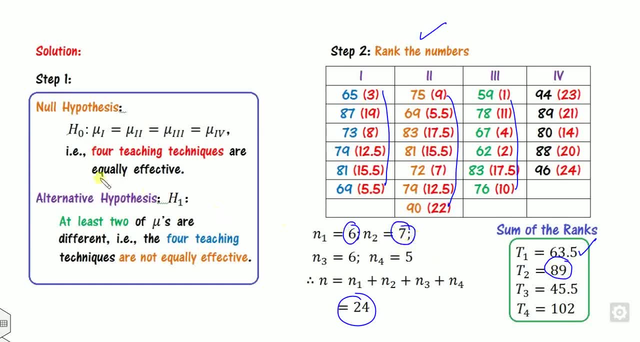 63.5 square divided by six plus 63.5 square divided by six plus what is the n2 is: t2 is 89 and what is the n2 is: t2 is 89 and what is the n2 is: t2 is 89 and it's seven, so this is 89 square. 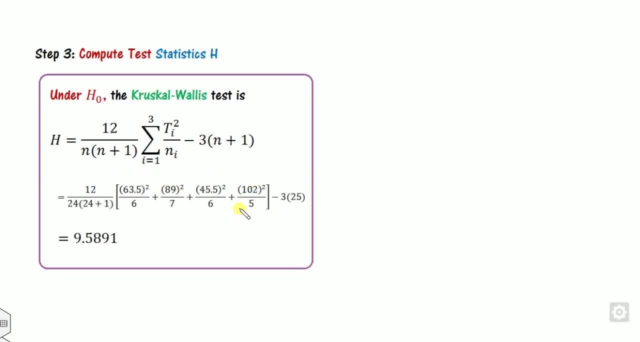 it's seven, so this is 89 square it's seven, so this is 89 square plus seven, and so on. you will calculate plus seven, and so on. you will calculate plus seven, and so on. you will calculate the values as the values, as the values, as here now. the stop last step is step number. 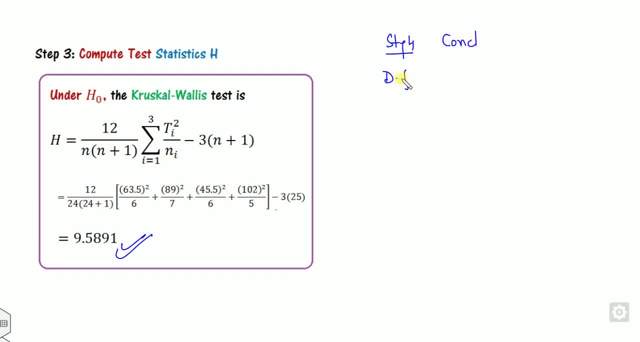 here now the stop last step is step number. here now, the stop last step is step number. four is a conclusion. four is a conclusion. four is a conclusion. what is the degree of freedom is df what? what is the degree of freedom is df what? what is the degree of freedom is df? what is the meaning of the df is? 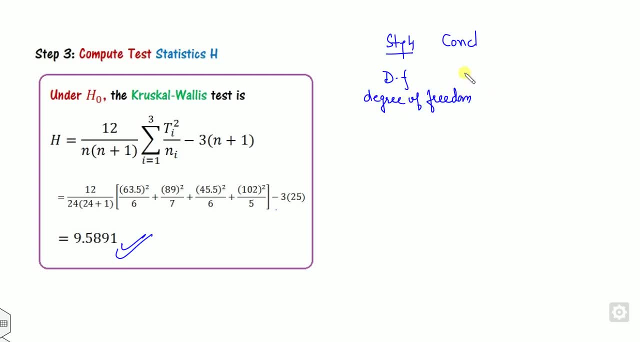 is the meaning of the df is? is the meaning of the df is degree of freedom. so what is the degree? degree of freedom. so what is the degree? degree of freedom. so what is the degree of freedom? is k minus one how many of freedom? is k minus one, how many? 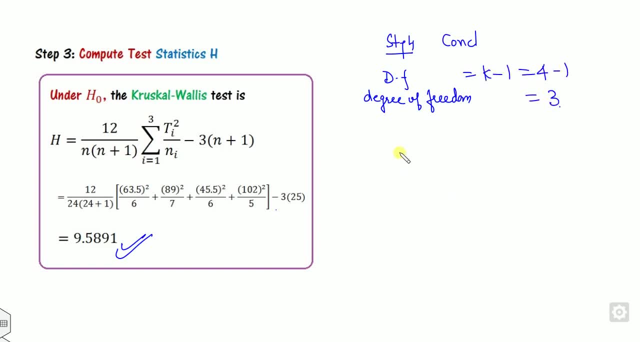 of freedom is k minus one. how many samples are there? four, four minus one is samples. are there four? four minus one is samples. are there four? four minus one is three. so you need the tabulated value of three. so you need the tabulated value of three. so you need the tabulated value of the chi square with a three degree of. 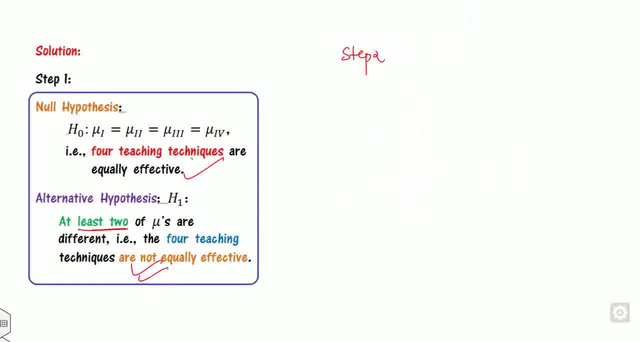 the chi square with a three degree of the chi square, with a three degree of freedom: freedom, freedom and level of significance is given to you and level of significance is given to you and level of significance is given to you. let me check in the question. yes, it's a. 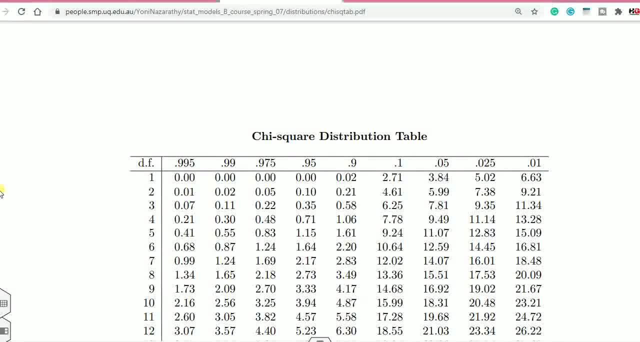 let me check in the question. yes, it's a. let me check in the question. yes, it's a five percentage. so what is the value of five percentage? so what is the value of five percentage? so what is the value of the, the, the three degree of freedom, this is the. 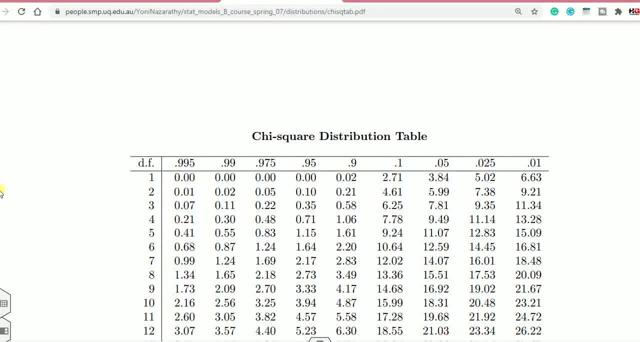 three degree of freedom. this is the three degree of freedom. this is the three level of significance. five is 7.81. three level of significance: five is 7.81. three level of significance: five is 7.81. so you can see, you can write here as: 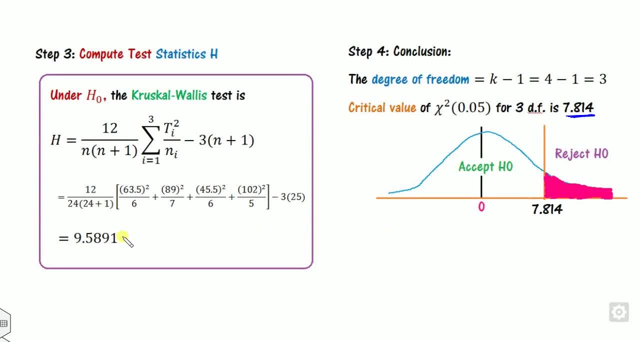 so you can see you can write here as: so you can see you can write here as: value as 7.814. value as 7.814. value as 7.814. now look at this value is lies in which: now look at this value is lies in which 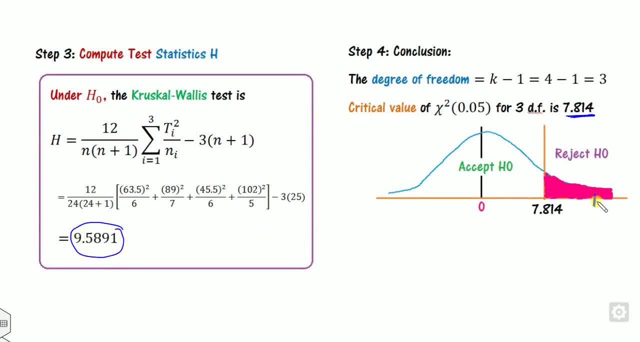 now look at this. value is lies, in which case it lies here. so h0 is rejected- case it lies here. so h0 is rejected- case it lies here. so h0 is rejected. so what is the h0? is all the teaching. so what is the h0? is all the teaching. 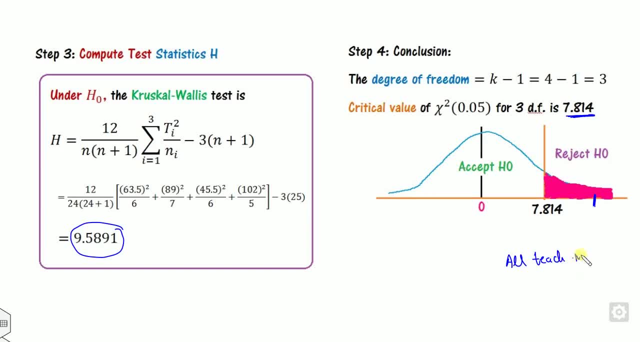 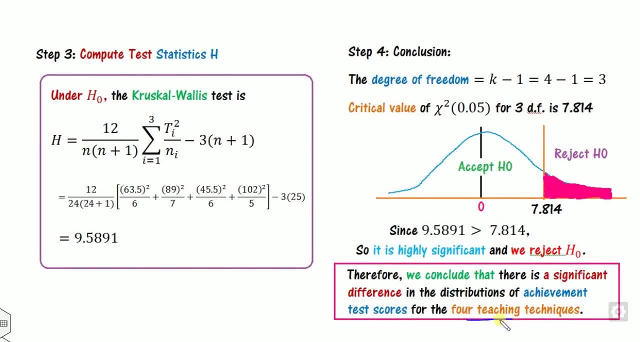 so what is the h0? is all the teaching methods, are methods, are methods, are all the teaching methods are same. so all the teaching methods are same. so all the teaching methods are same. so that is rejected. so that is rejected. so that is rejected. so it means the teaching methods are not. 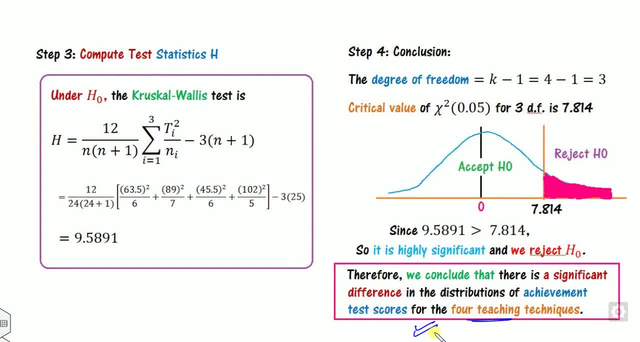 it means the teaching methods are not. it means the teaching methods are not same or entirely same, or entirely same or entirely different, different, different. so this is a simple procedure you can. so this is a simple procedure you can. so this is a simple procedure you can apply to solve the crucial values test. 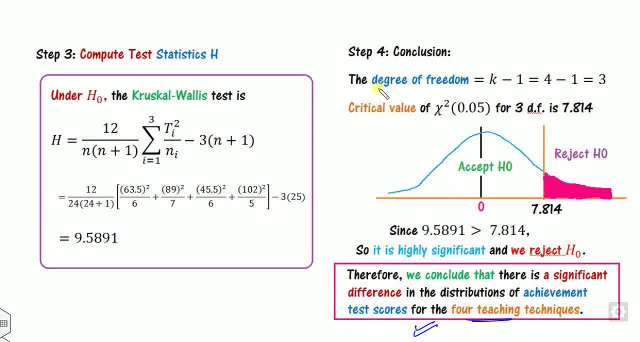 apply to solve the crucial values test. apply to solve the crucial values test. or this is analog to the one way: anova. or this is analog to the one way: anova. or this is analog to the one way: anova. so always remember, student, this is the. 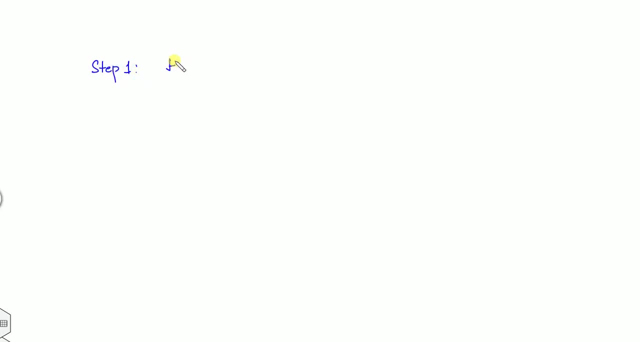 so always remember student. this is the. so always remember student. this is the four step rule, four step rule, four step rule. i can quickly recall that what is the? i can quickly recall that what is the? i can quickly recall that what is the step one is define h0, h1. 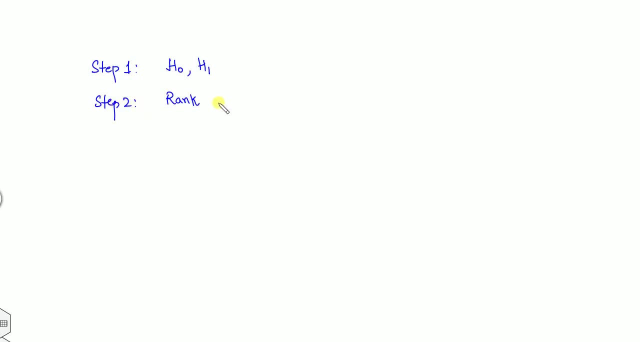 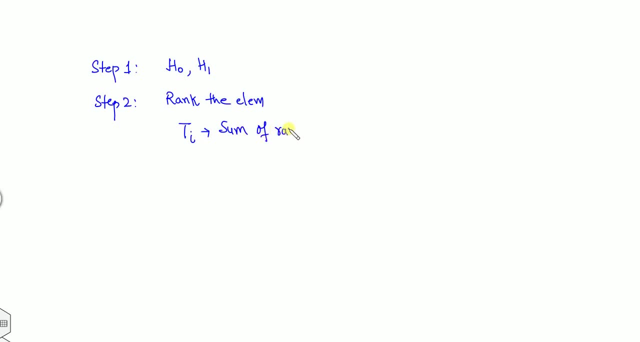 and then you have to find the ti's, and then you have to find the ti's sum of the ranks, and then you have to find the ti's sum of the ranks, and then you have to find the ti's sum of the ranks. sample wise. sample wise. 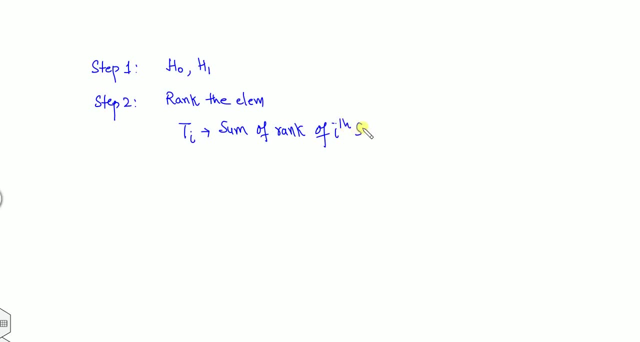 sample. wise, you have to find the sum of the ranks of. you have to find the sum of the ranks of. you have to find the sum of the ranks of the ith sample, the ith sample, the ith sample. once you define this, then step third is: once you define this, then step third is: 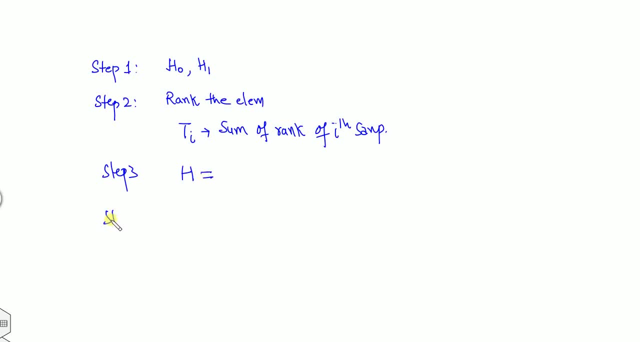 once you define this, then step third is: you have to find the value of the h, you have to find the value of the h, you have to find the value of the h, and then step four is: you have to find. and then step four is you have to find. 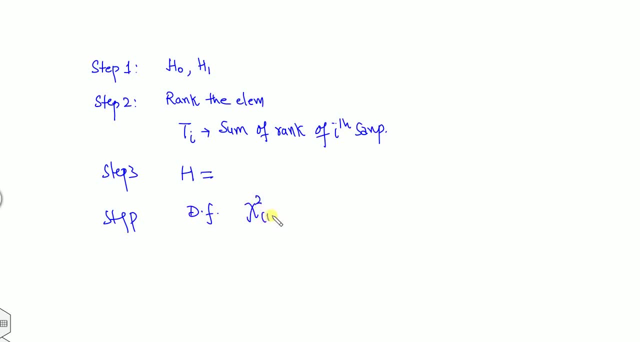 and then step four is: you have to find the degree of freedom, the degree of freedom, the degree of freedom, and find the value of the chi square with, and find the value of the chi square with, and find the value of the chi square with the k minus one degree of freedom. 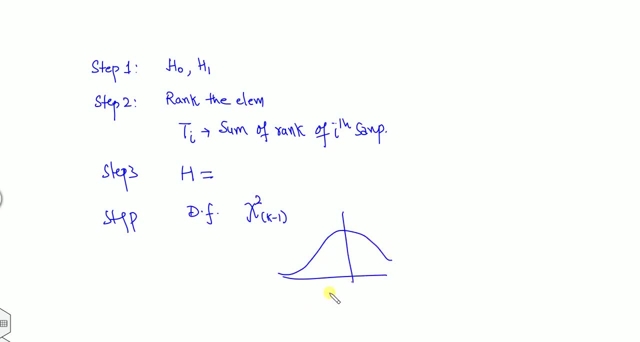 the k minus one degree of freedom, the k minus one degree of freedom, and finally make the conclusion, and finally make the conclusion and finally make the conclusion. so this is a simple procedure of the. so this is a simple procedure of the. so this is a simple procedure of the h test, or called as the crucial values. 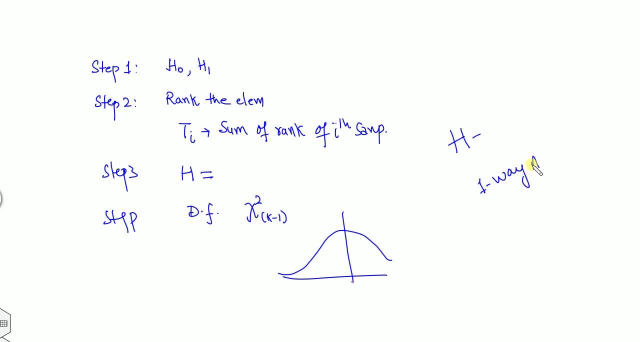 h test, or called as the crucial values. h test, or called as the crucial values, that is for the, that is for the. that is for the one way anova. this is a supplement of the one way anova. this is a supplement of the one way anova. this is a supplement of the one-way anova in the non-parametric test. 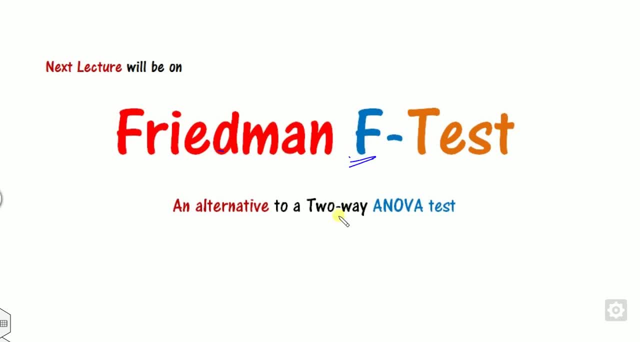 one-way anova in the non-parametric test. one-way anova in the non-parametric test. we will see in the next class. that is a we will see in the next class. that is a we will see in the next class. that is a fireman f test, which is the analog of